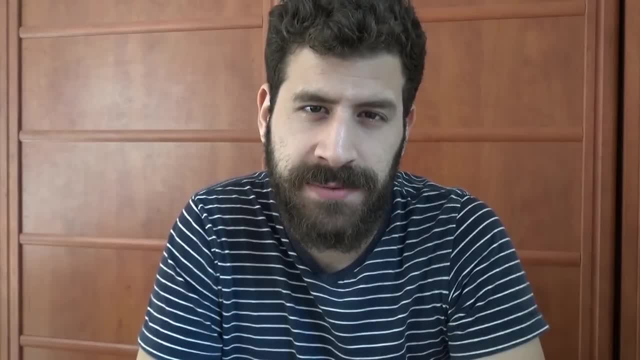 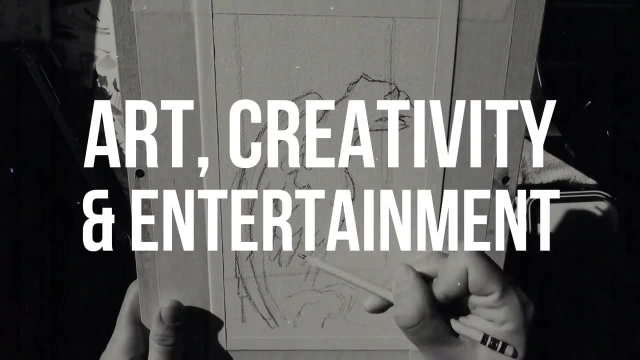 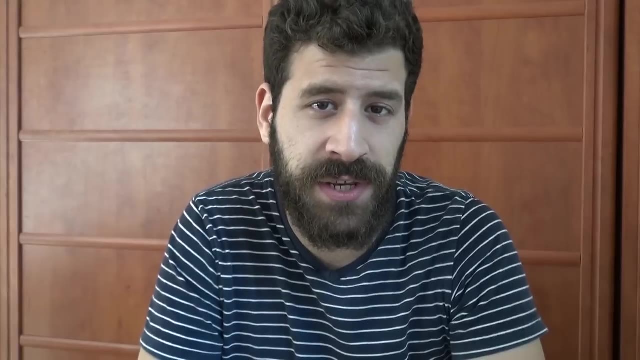 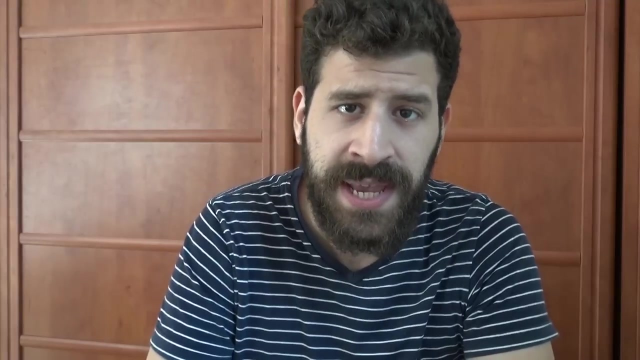 Today we're sketching three-dimensional shapes. What up friends, Liron here, Thank you for joining me in another video. Today. I want to do something a little special, So I want us to work together on sketching three-dimensional shapes, and I'm 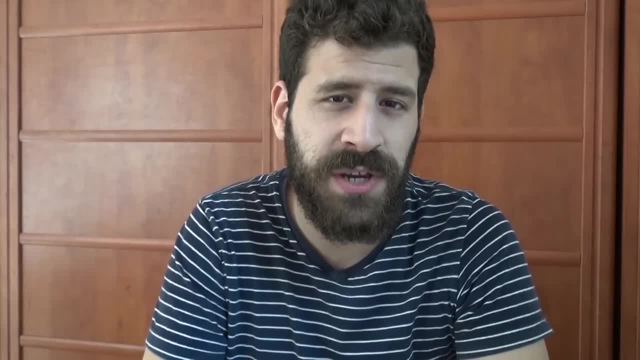 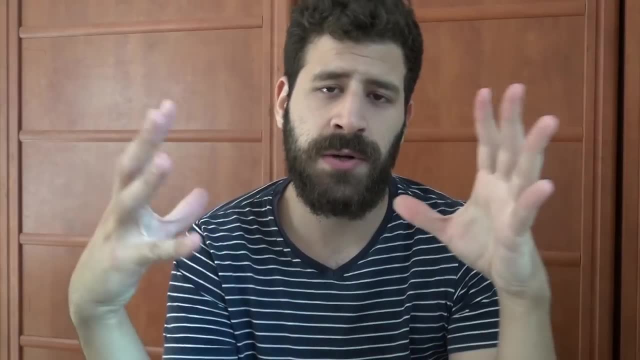 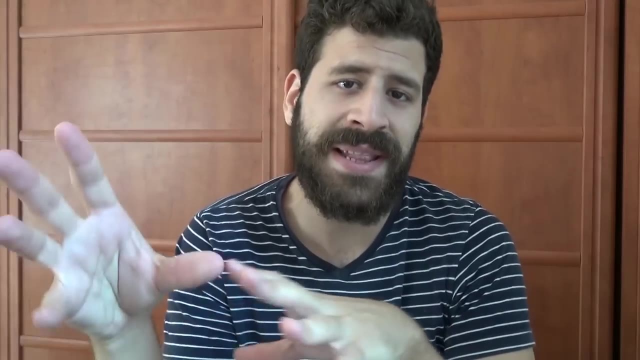 going to make it a little interesting, because there are quite a few videos out there on drawing cubes and pyramids and ovals and things like this. They talk about how to create a sense of depth and three-dimensionality. So we're gonna go a bit over that, But then I want to share with 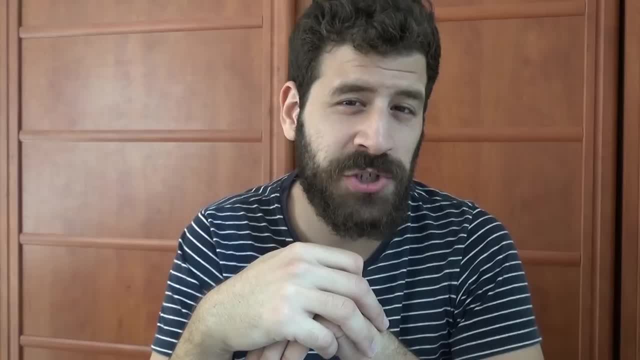 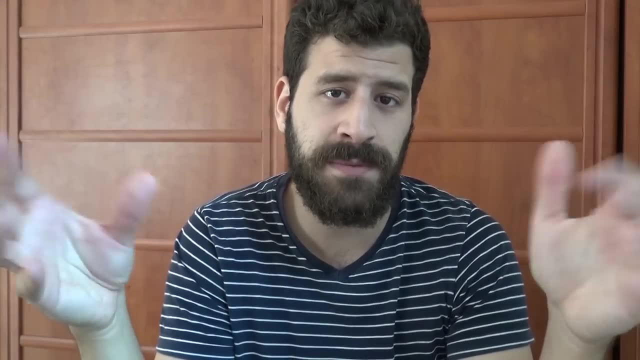 you a funny sort of exercise or doodle session that I used to do with myself just since I was really young, And I just intuitively did it because I enjoyed it, But when I thought back at it it really improved my visual perception and skills And it's just something so 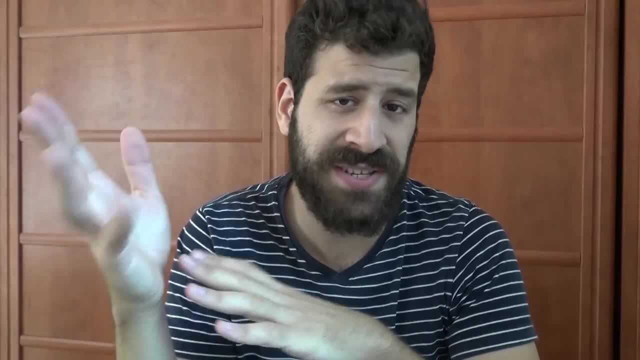 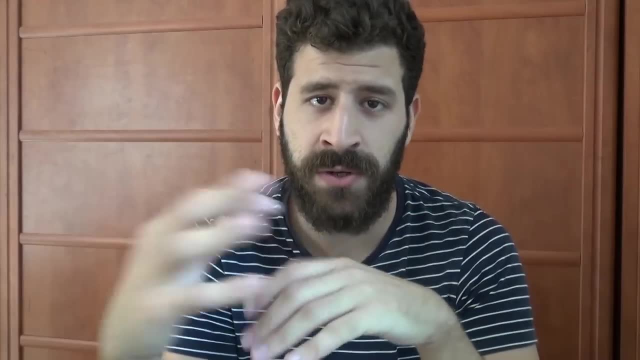 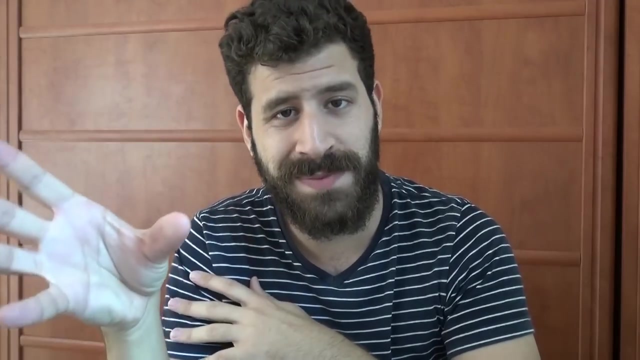 simple that anyone can do it. It's a simple exercise that anyone can do and just really improve the way you perceive objects and your ability to rotate them in mind. okay, Now I'm gonna do quite a bit in this video, So if you want me to focus on a specific topic in the future, 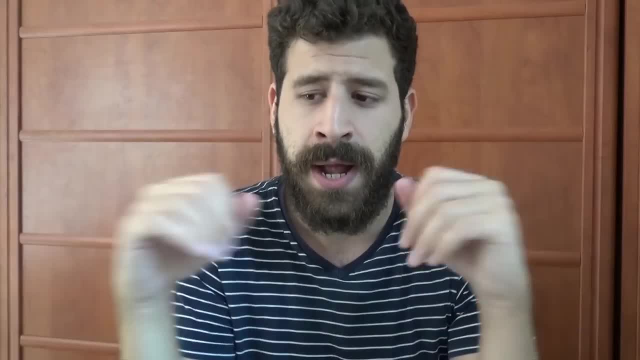 let me know in a comment below. I know I'm kind of all over the place, But then I think it wraps up nicely And then we can, I think, zoom in on a specific topic if you want to. okay, So don't. 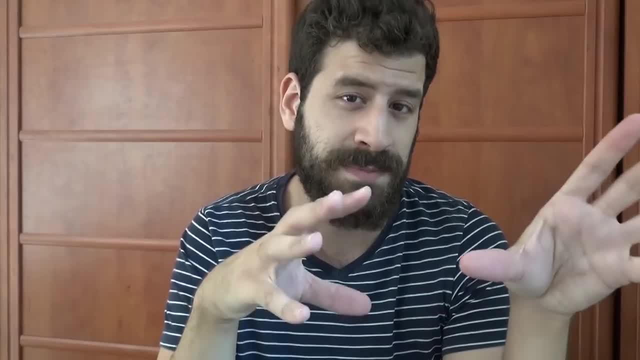 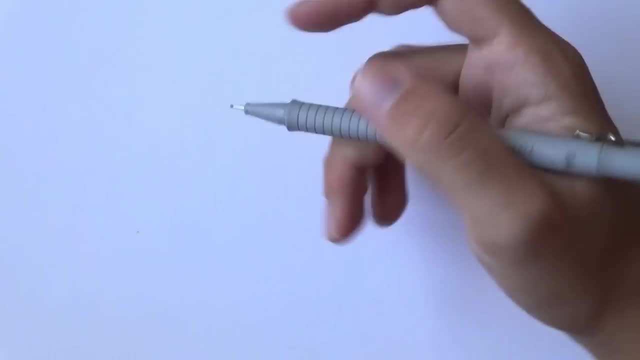 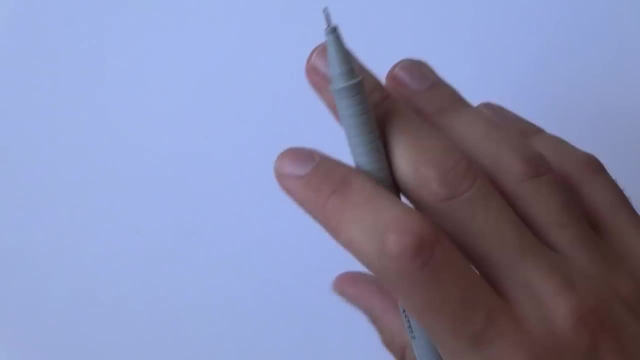 forget to leave it in a comment below if you want me to focus on something specific. And, with that being said, let's get started. Okay, so let's get started. And the goal here is to really just have fun and sort of practice- our ability to understand three-dimensional shapes and draw them. okay, I'll. 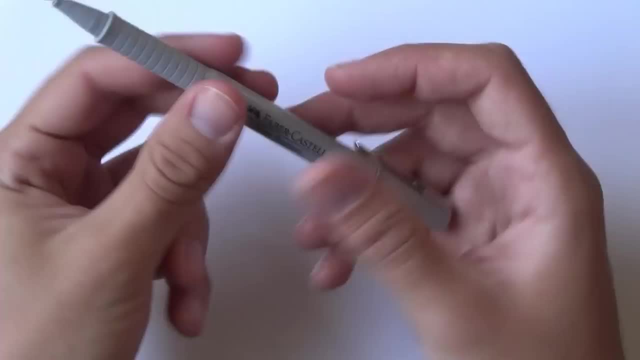 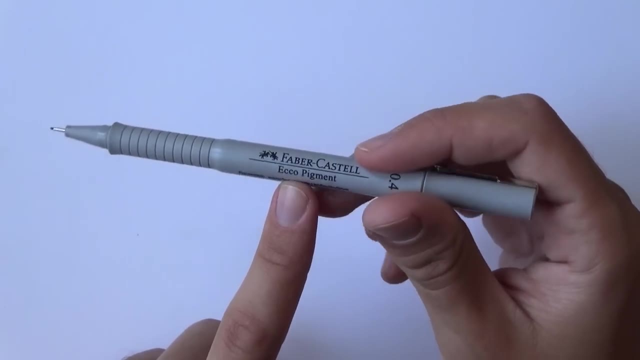 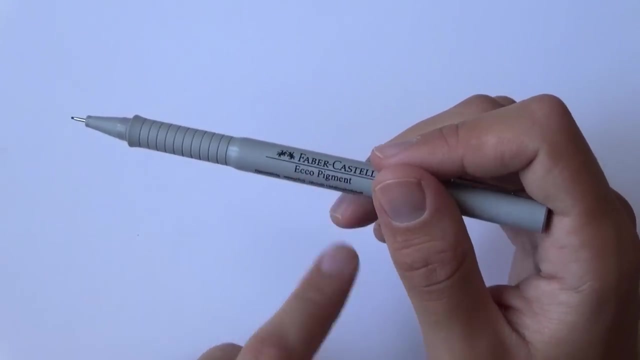 be using the new Faber-Castell pen. I do need to, and some of you mentioned in the comments. I do still need- to demonstrate sort of a water resistance or waterproof test with watercolor, just so that we can better know if this can really endure watercolor. But that's for another video. You 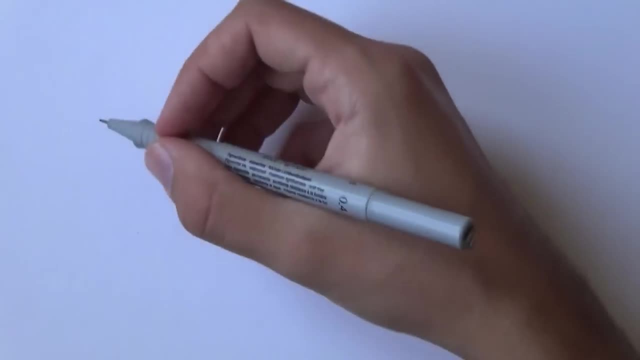 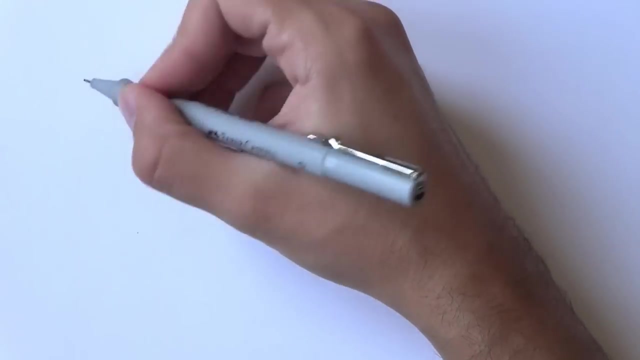 can use a pen or anything, a pencil or anything else you want. I'll be working with a pen, Okay? so basically, the simplest three-dimensional shape that you can create is just sort of a ball, okay. So in this case we have this sort of a ball and it's just a circle Now without 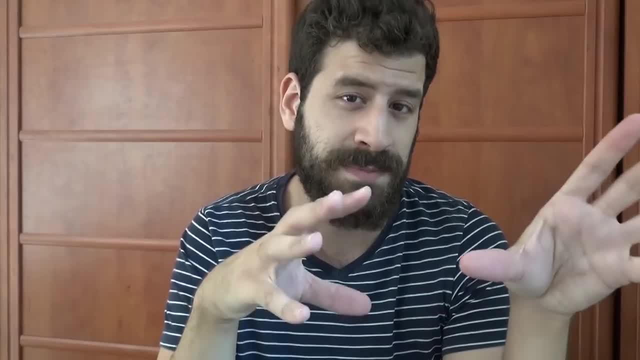 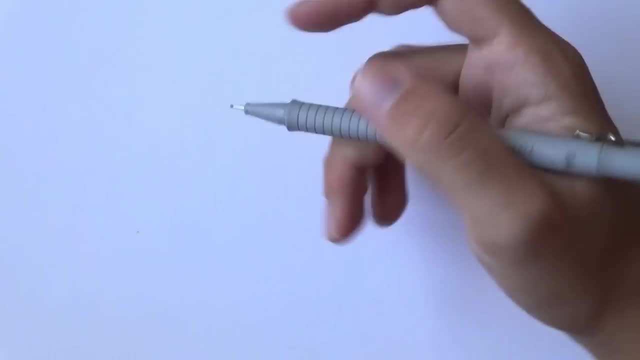 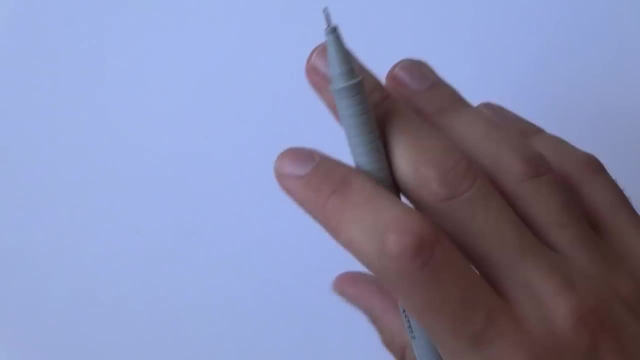 forget to leave it in a comment below if you want me to focus on something specific. And, with that being said, let's get started. Okay, so let's get started. And the goal here is to really just have fun and sort of practice- our ability to understand three-dimensional shapes and draw them. okay, I'll. 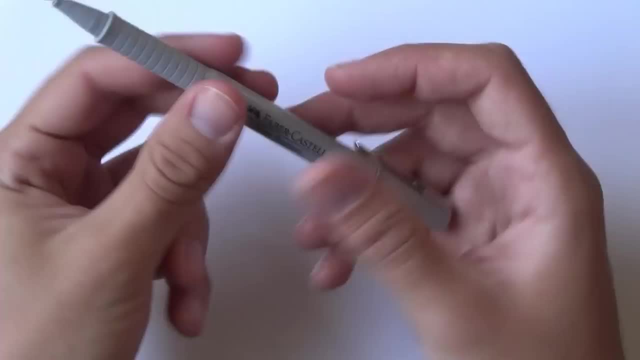 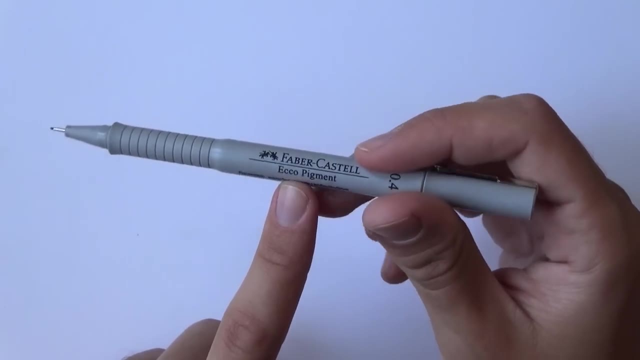 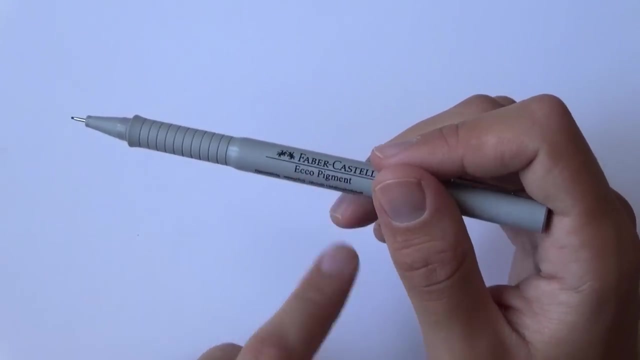 be using the new Faber-Castell pen. I do need to, and some of you mentioned in the comments. I do still need- to demonstrate sort of a water resistance or waterproof test with watercolor, just so that we can better know if this can really endure watercolor. But that's for another video. You 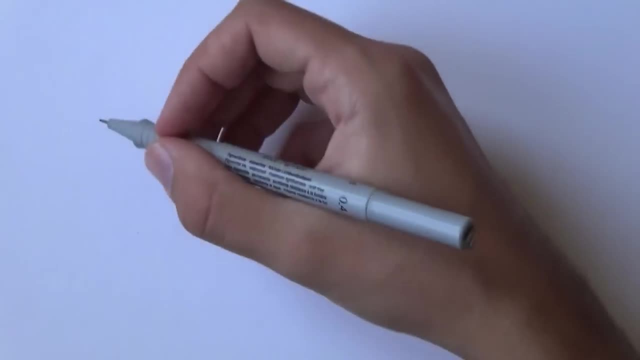 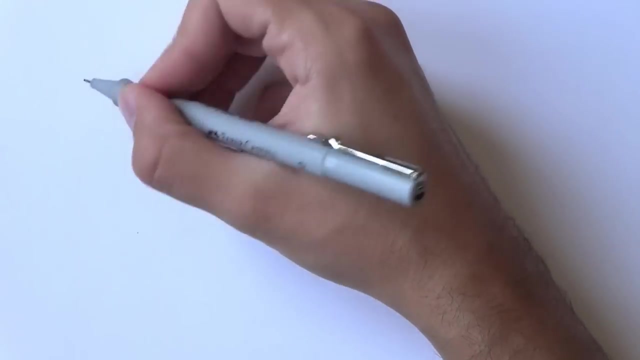 can use a pen or anything, a pencil or anything else you want. I'll be working with a pen, Okay? so basically, the simplest three-dimensional shape that you can create is just sort of a ball, okay. So in this case we have this sort of a ball and it's just a circle Now without 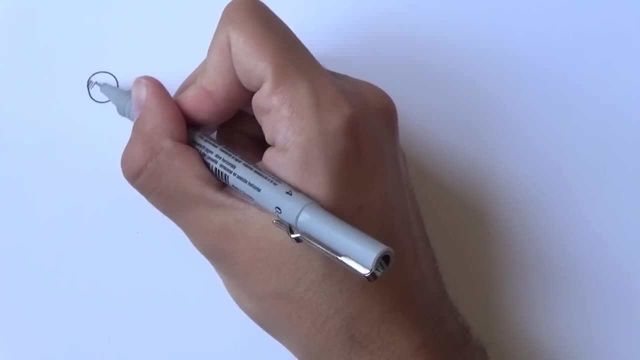 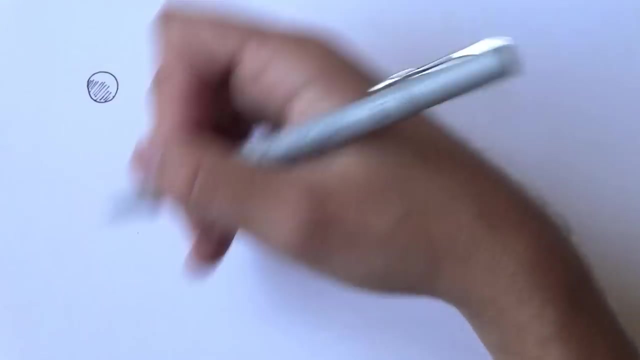 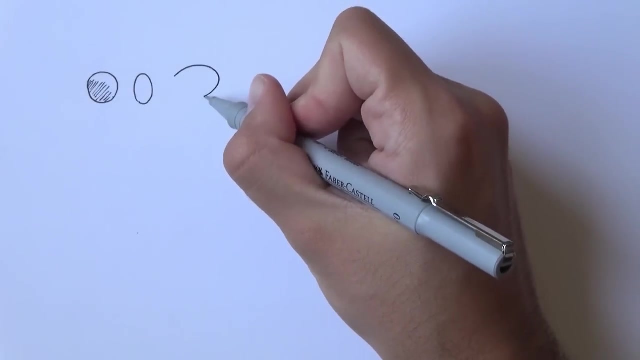 any shadows or anything. it's not even a ball, So I'm just gonna add a small shadow here to the side. okay, But this is not really that interesting. You know, you can play around with it and create sort of an egg-like shapes, sort of ellipses or ovals, which is nice, but that's not really. 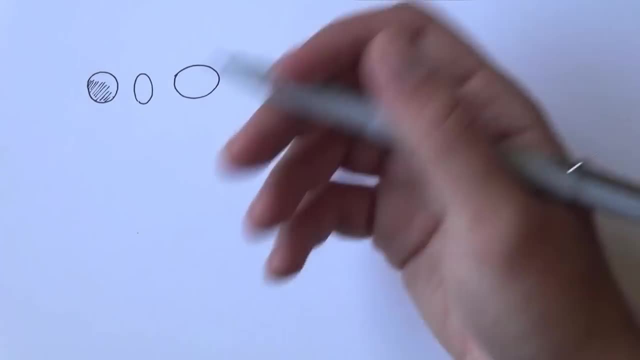 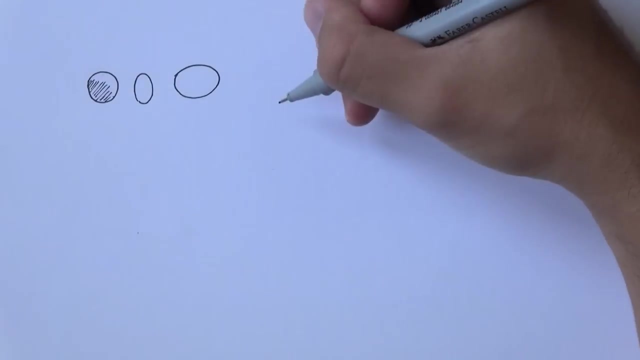 too interesting. So what I want to work on is just the next kind of best thing, And the easiest shape is a cube. Now, the cube is very simple. I actually did a few videos on that, but the cube is very simple to draw. So basically, it's like drawing the simplest way of drawing. it is just if you. 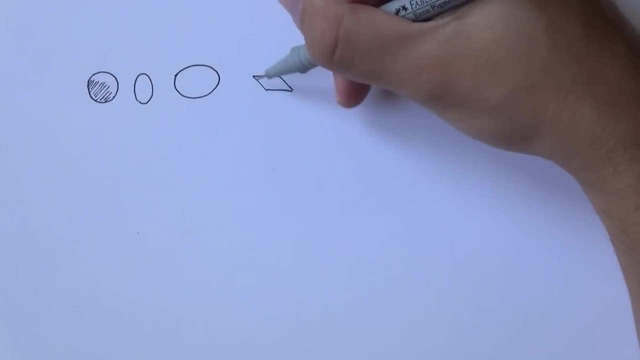 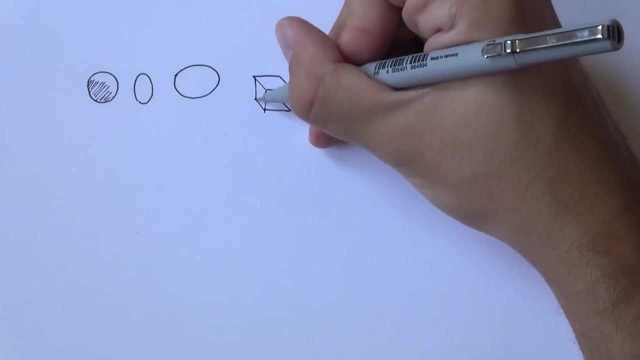 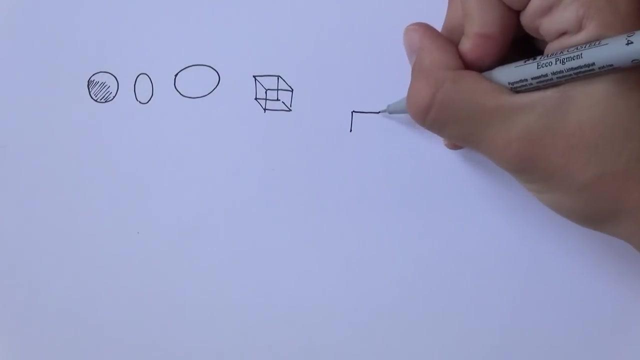 draw two kind of parallelograms or a trapezoid or whatever you want to call that shape, kind of like this, And then you sort of connect all of the corners and then you get a transparent cube. okay, There's tons of ways to do this. You can just sort of draw a square. 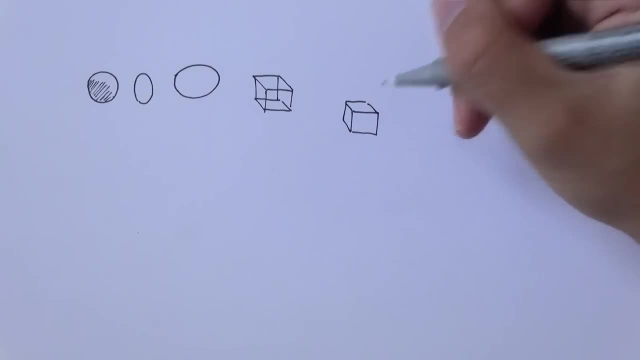 then pull vertical lines, connect them and you get a cube. Now where the real value comes from is practicing drawing the cube in many different angles. okay, So if we look at the cube straight from the front like this, the way the arrow indicates what we will get is just a square. 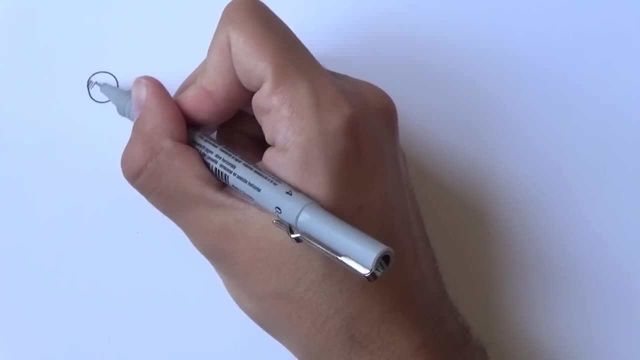 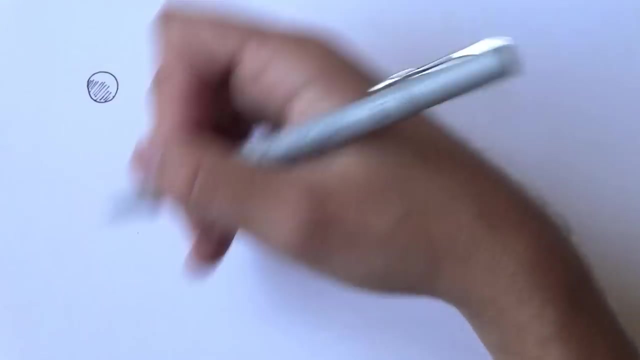 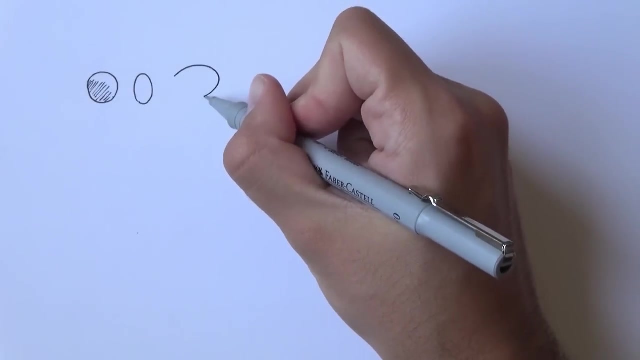 any shadows or anything. it's not even a ball, So I'm just gonna add a small shadow here to the side. okay, But this is not really that interesting. You know, you can play around with it and create sort of an egg-like shapes, sort of ellipses or ovals, which is nice, but that's not really. 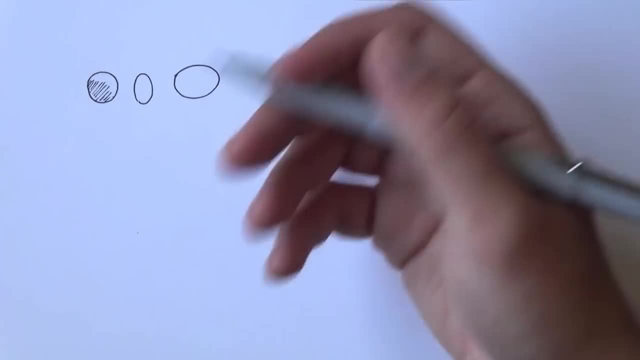 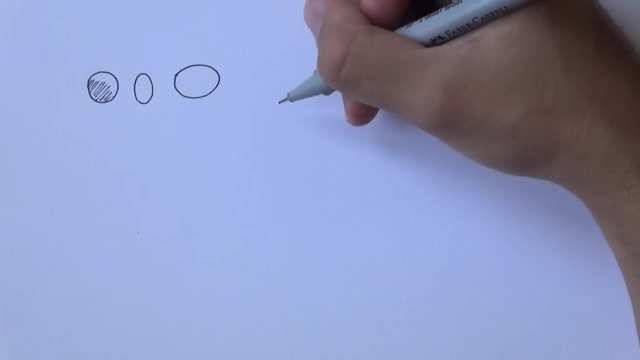 too interesting. So what I want to work on is just the next kind of best thing, And the easiest shape is a cube. Now, the cube is very simple. I actually did a few videos on that, but the cube is very simple to draw. So basically, it's like drawing the simplest way of drawing. it is just if you draw. 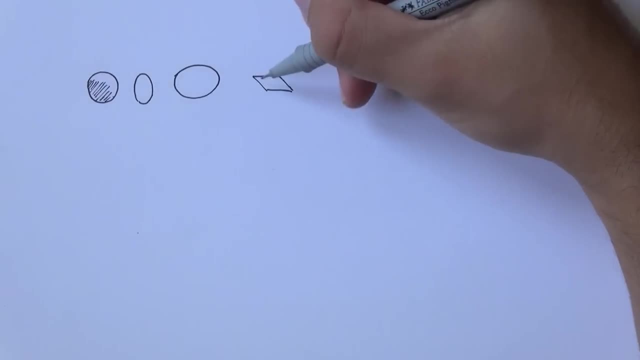 two kind of parallelograms or trapezoid or whatever you want to call that shape, kind of like this, And then you sort of connect all of the corners and then you get a transparent cube. okay, There's tons of ways to do this. You can just sort of draw a square. 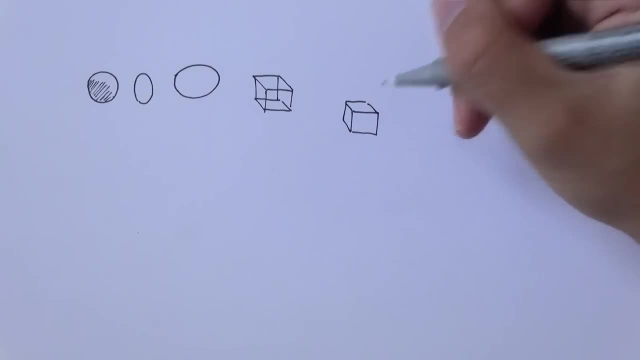 then pull vertical lines, connect them and you get a cube. Now where the real value comes from is practicing drawing the cube in many different angles. okay, So if we look at the cube straight from the front like this, the way the arrow indicates what we will get is just a square. 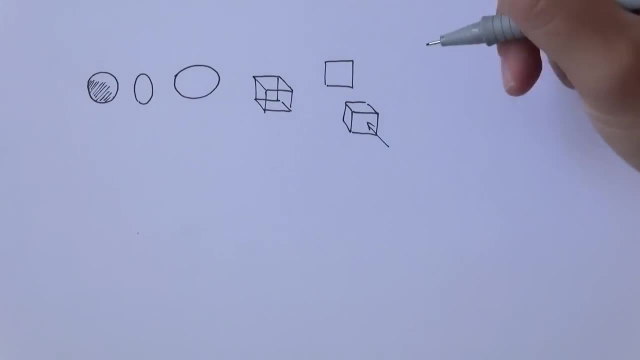 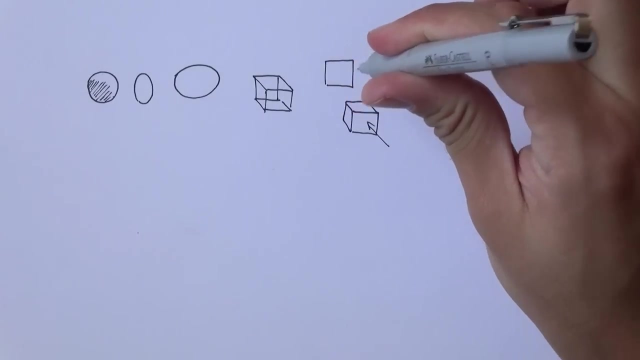 okay, Like this, Or sort of a rectangular, depending on the cube. Now, if we look a bit more from the right- so think about it this way- We're looking at it dead on- If we look a bit to the right, we're gonna see a little bit more of its right side. okay, And this is what I want to. 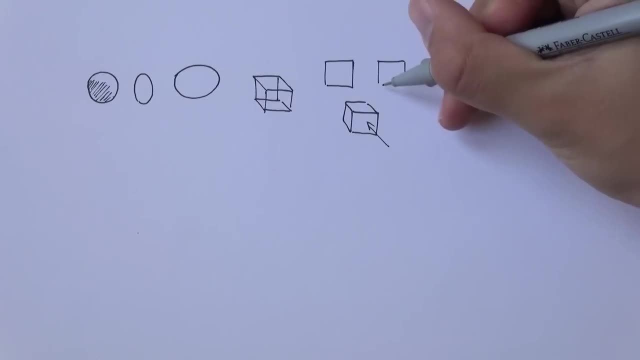 show you now. So we still have that kind of a square shape, but now we can see a bit of its right side. okay, Now, the more we turn it, the less we're gonna see from the front and the more we're gonna. 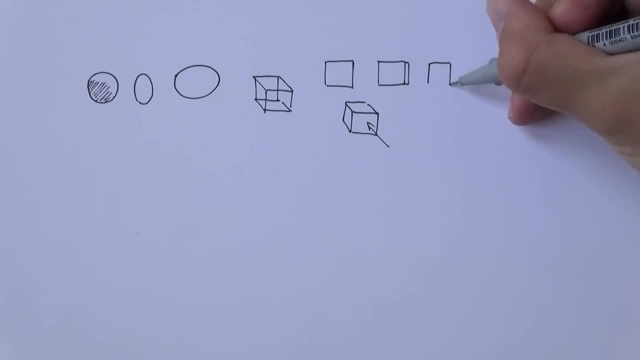 see from the side. So we have sort of a little bit less of this and a little bit more of the side, okay, And the more we turn it, we will get much less from the left side and more of the right side. okay, So if this is the 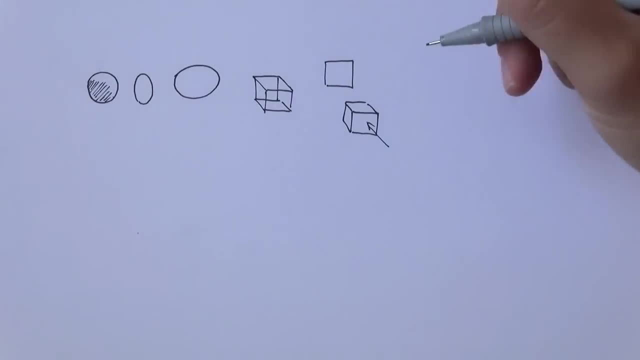 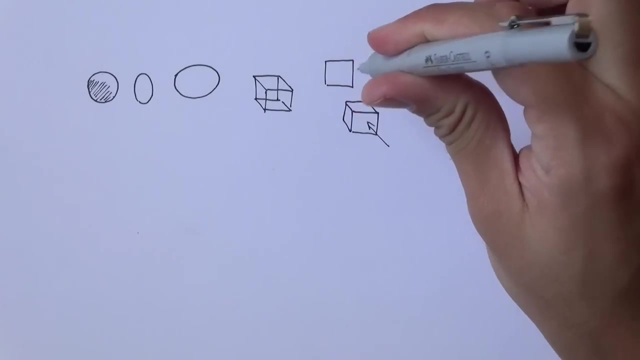 okay, Like this, Or sort of a rectangular, depending on the cube. Now, if we look a bit more from the right- so think about it this way- we're looking at it dead on. If we look a bit to right, we're going to see a little bit more of its right side. okay, And this is what I want to show. 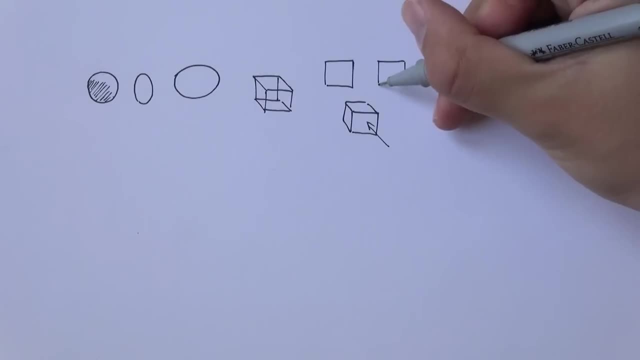 you now. So we still have that kind of a square shape, but now we can see a bit of its right side. okay, Now, the more we turn it, the less we're going to see from the front and the more we're going to see from the side. So we have sort of a little bit less of this and a little bit more of. 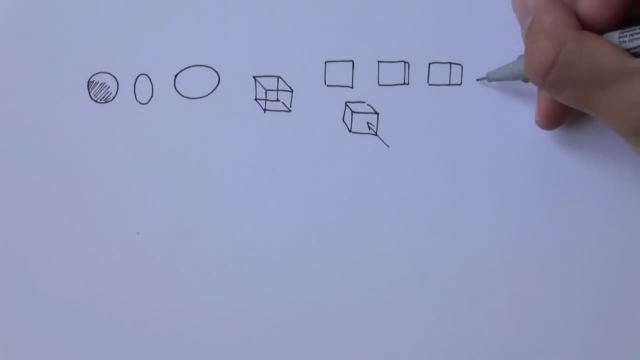 this side, okay, And the more we turn it, we will get much less from the left side and more of the right side, okay. So if this is the right side, let me just put in some sort of a shadow on it, just to better indicate where it is. 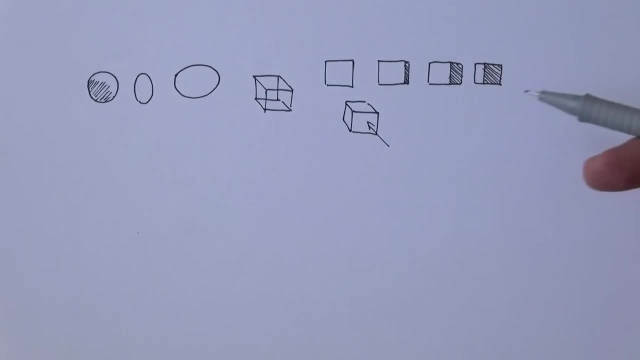 okay, And you can see it's sort of: the more we look from the right, the more we see this side. Now let's take into consideration also looking from above. So if we'll take this cube and we'll just look at it from above, we're going to see a bit more of the top plane, okay, So this is. 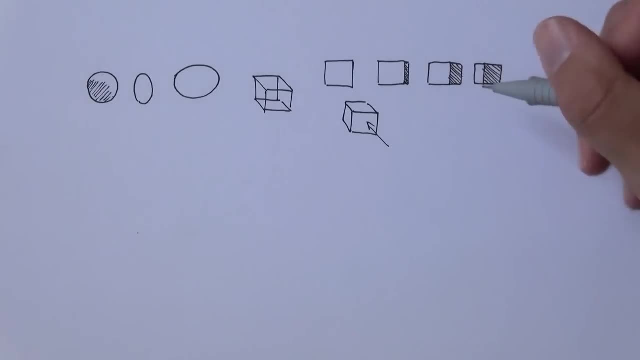 what I want to do now. So I'm just going to do it a little larger. this is sort of an intro. Now we're going to make it a little larger. So, basically, to get a better view of the top, this line is going to have to be squeezed and not be. 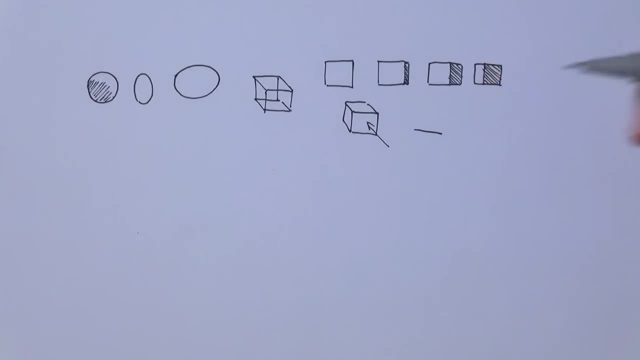 completely horizontal but rather a bit diagonal. okay, Then this line, same thing. it's going to be a bit of an angle like this, And now we get to see, using parallel lines to this one and parallel lines to this one, we get to see a bit of the top. okay. 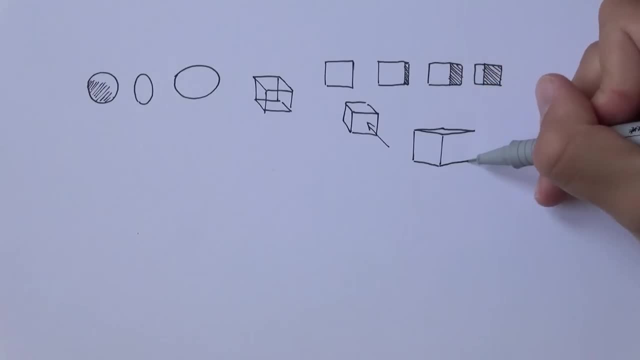 And we can also see that left side and the right side. okay, And this is the right side. from earlier on that I kept sort of darkening this side, And the more we change our angle, the more we're going to see of that top plane, okay, So if we look more from above, 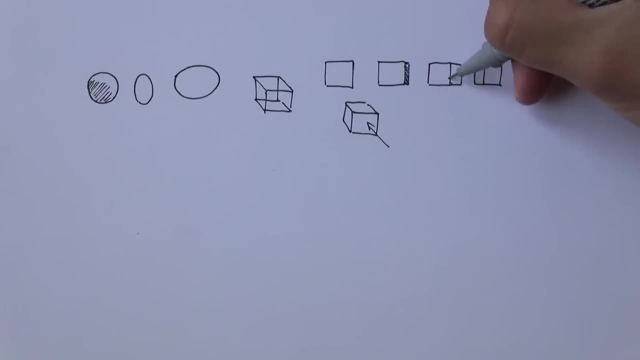 right side. let me just put in some sort of a shadow on it just to better indicate where it is Okay And you can see. it's sort of: the more we look from the right, the more we see this side. Now let's take into consideration also looking from above. So if we'll take this here and we'll 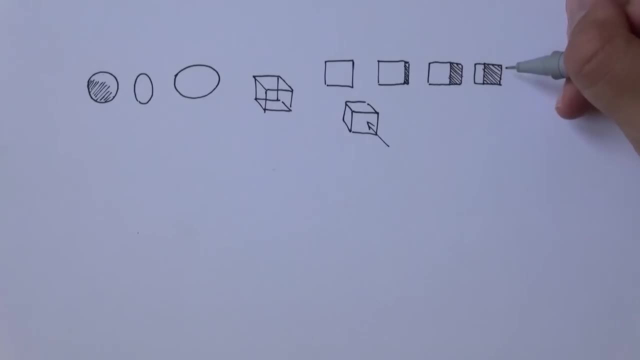 just look at it from above, we're gonna see a bit more of the top plane, Okay, so this is what I wanna do now. So I'm just gonna do it a little bit further from the moving side, little larger. just this is sort of an intro. now we're going to make it a little larger, so basically, 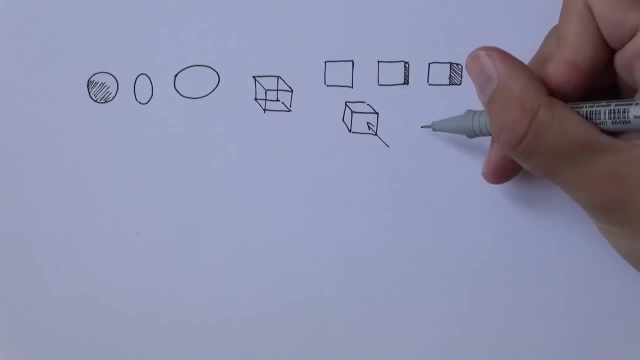 to get a better view of the top. this line is going to have to be squeezed and not be completely horizontal but rather a bit diagonal. okay, then this line, same thing. it's going to be a bit of an angle like this, and now we get to see, using parallel lines to this one and parallel 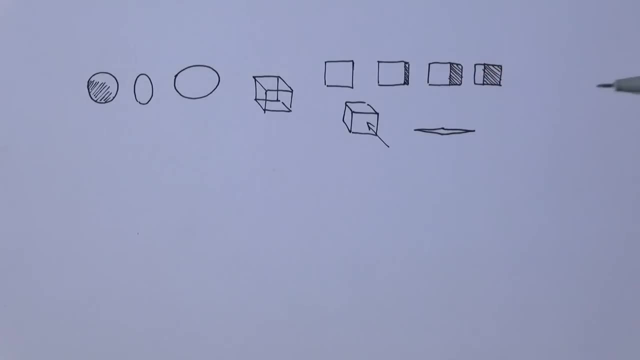 lines to this one, we get to see a bit of the top, okay, and we can also see that left side and the right side, okay, and this is the right side. from earlier on that i kept sort of darkening this side, and the more we change our angle, the more we're going to see of that top plane. okay, so if 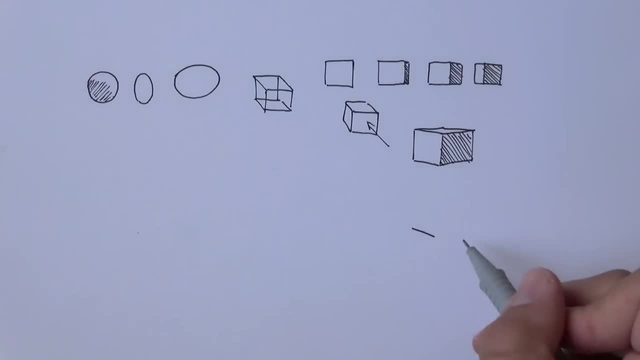 we look more from above. this line is going to be even more diagonal, and this line also is as well. it's going to be a little more diagonal, and then you get, you get a little more diagonal, and then you get a little more diagonal, and then you get a little. 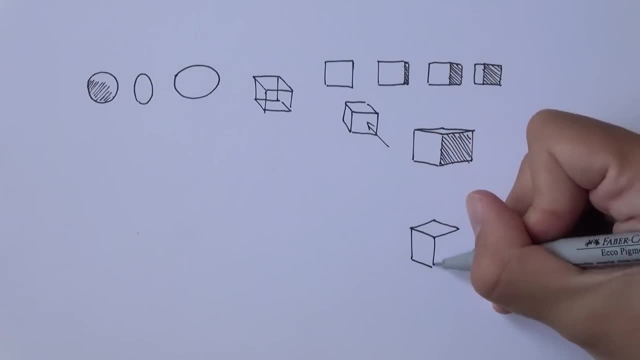 this sort of a cube look, and i think a really good exercise will be just to try out as many variations as possible, maybe even putting it in perspective. so if you have one point, perspective meaning we get closer to the cube enough so that the distance of us from this area will be. 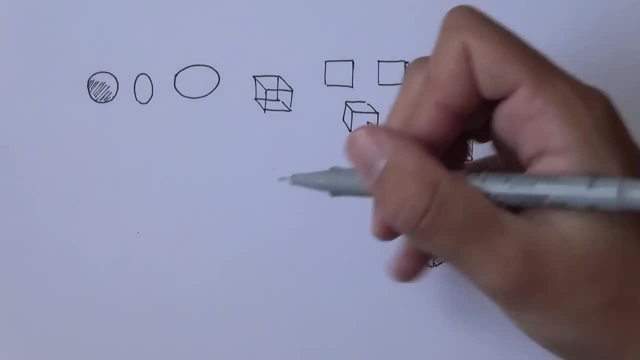 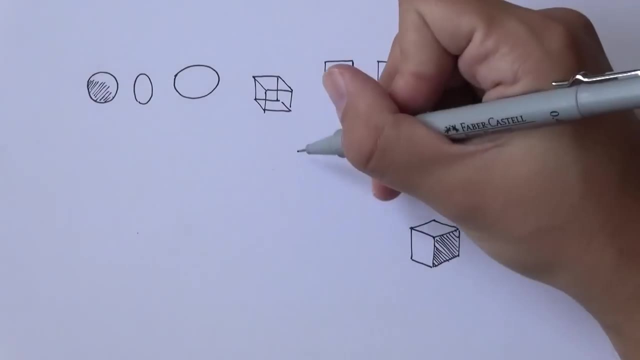 significantly different from this area, what happens in this example- and i will make a more detailed video about that because that's going to be a little bit more detailed- but i'm going to show you because that's a bit of a more complex object. so if we look at a cube, let's say like, in this angle, 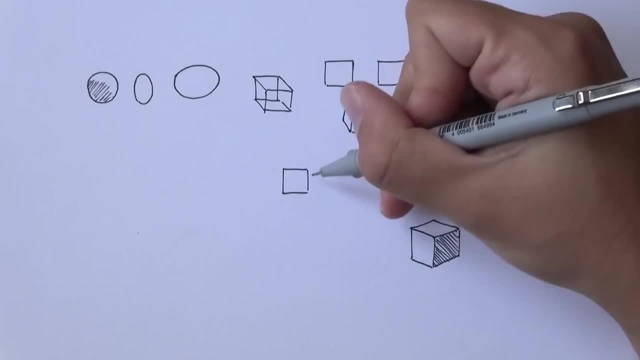 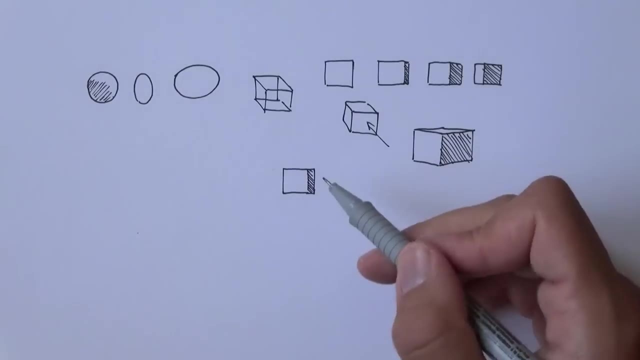 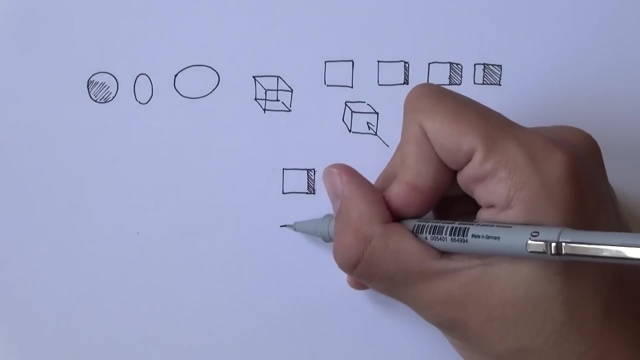 from far away it looks just like we did here. you have sort of a square and then the side side plane. but the closer we get to it, the more significant the difference in distance is between us and the front plane and the back side. so what will happen is that you'll sort of get a side that's moving. 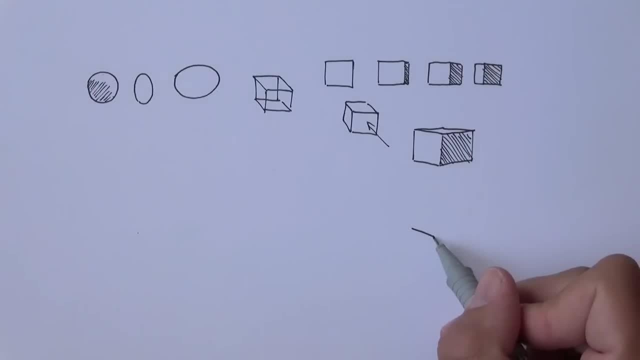 this line is going to be even more diagonal, and this line also, as well, is going to be a little more diagonal, And then you get this sort of a cube look, And I think a really good exercise will be just to try out as many variations as possible. 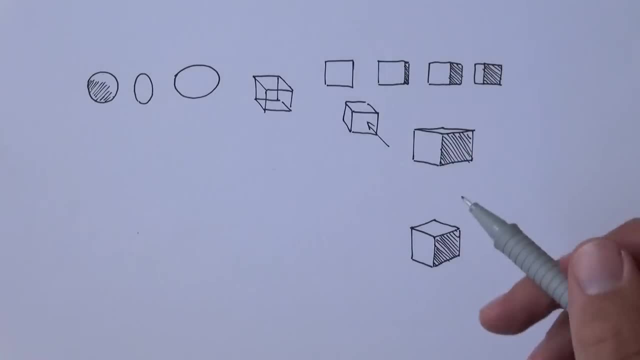 maybe even putting it in perspective. So, if you have one point, perspective meaning we get closer to the cube enough so that the distance of us from this area will be significantly different from this area. What happens in this example, and I will make a more detailed video- 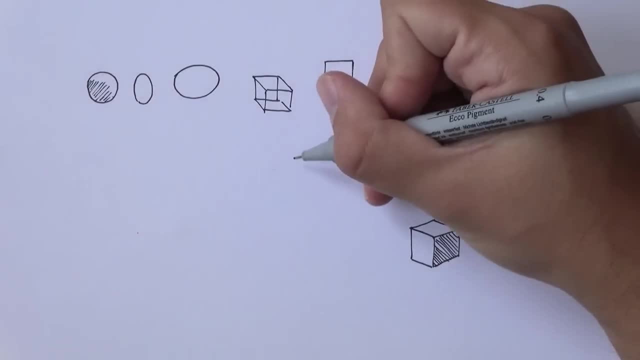 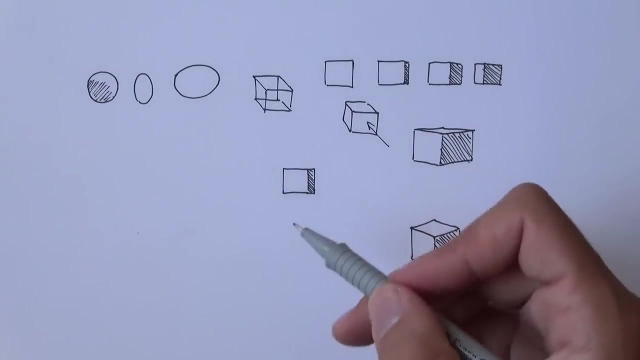 about that because that's a bit of a more complex object. So if we look at a cube this angle from far away, it looks just like we did here. you have sort of a square and then the side plane. But the closer we get to it, the more significant the difference in distance is between. 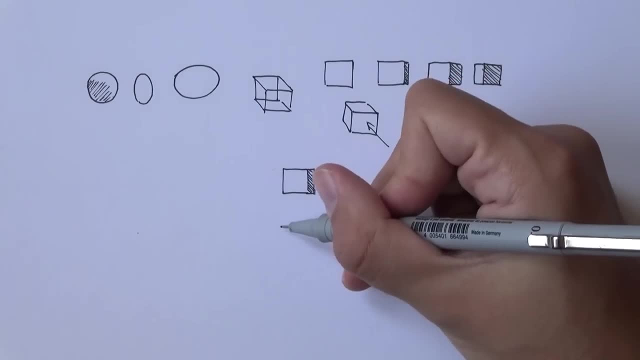 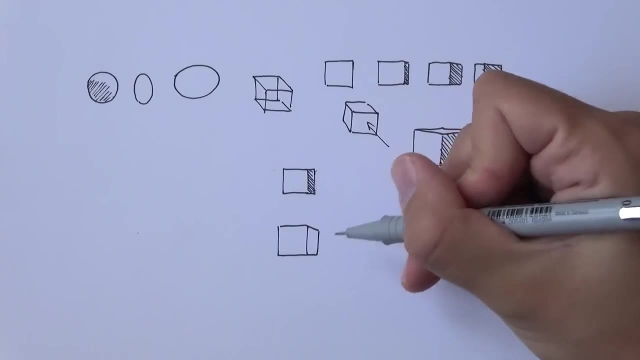 us in the front plane and the back side. So what will happen is that you'll sort of get a side that's moving towards a vanishing point, just like in the principles of perspective. okay, So you'll get this sort of a change in the way these lines work, And this is when I draw buildings. it's all based on that. 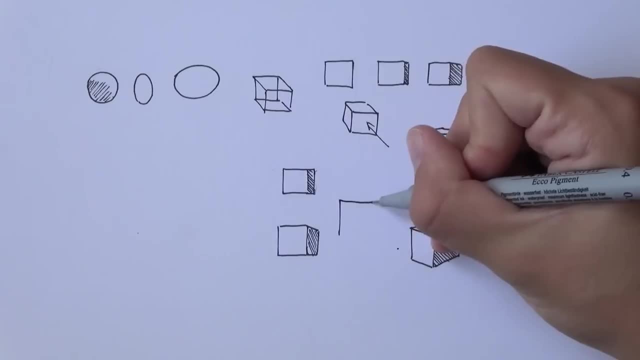 the more extreme it will get, the more you will see this. So let's just create another one for fun, And here we'll really put perspective into consideration, And you can see here sort of these lines move all towards this imaginary, imaginary vanishing point. is what? 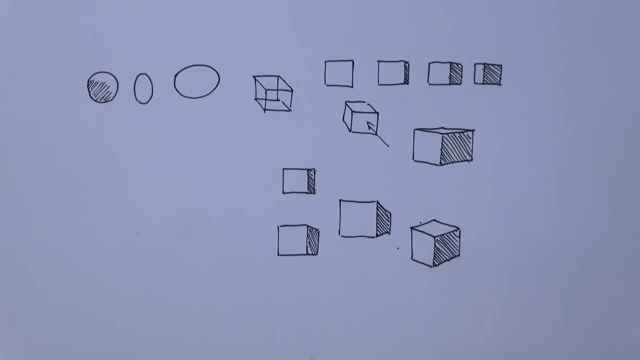 it's called Okay, and I will make a more detailed video about that. I promise Now this. so this for the key, And I think it's a really good exercise to play around with it. move it around, try and imagine it from different locations, from different angles, and maybe also working with a transparent cube. 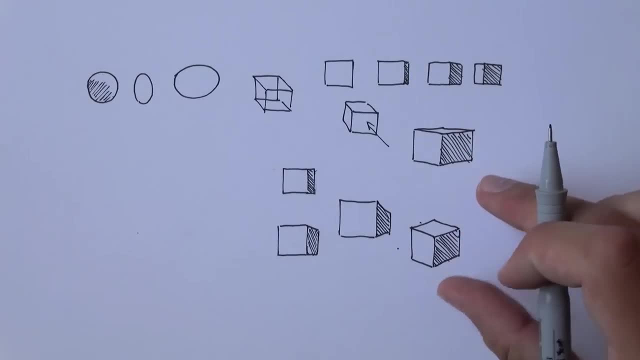 from time to time, So you can kind of turn it around in your head and try and draw it Now. you won't always succeed. It's not really easy if you don't have that sort of perception, But with practice you'll be able to do that. So this is for the cube. Now we have 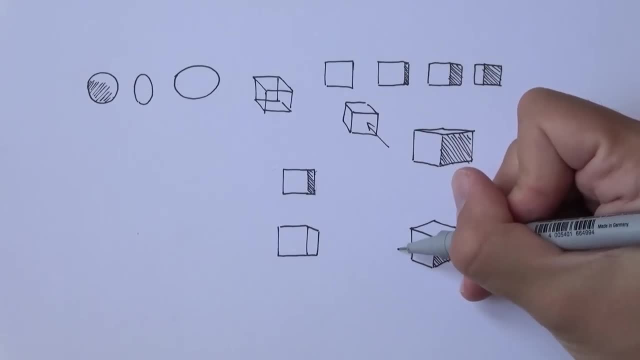 towards a vertical plane, and then you'll sort of get a side that's moving towards a vertical plane, and then you'll sort of get a side that's moving towards a vertical plane, and then you'll sort of get a vanishing point, just like in the principles of perspective. okay, so you'll get this sort of a. 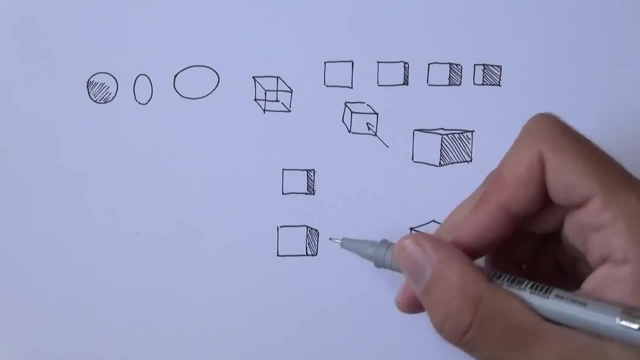 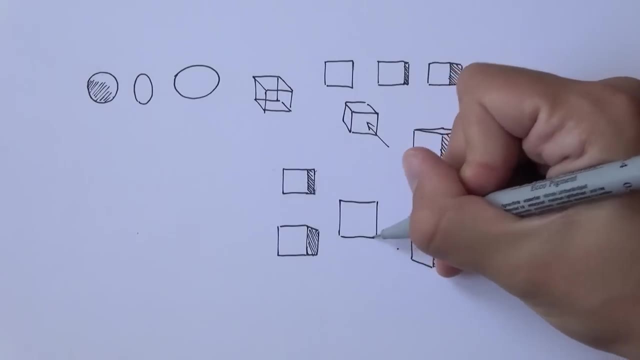 a change in the way these lines work, and- and this is when i draw buildings- it's all based on that the more extreme it will get, the more you will see this. so let's just create another one for fun, and here we'll really put perspective into consideration and you can see here sort of these. 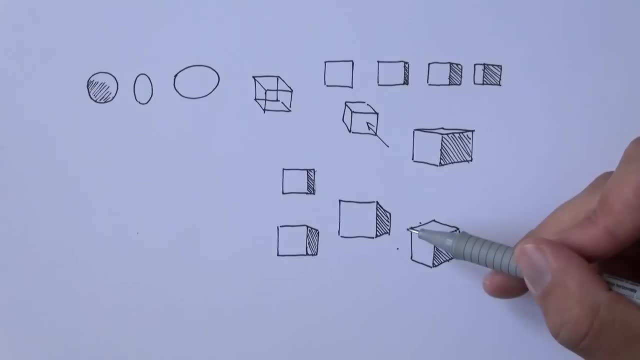 lines move all towards this imaginary- um, imaginary vanishing point is what it's called. okay, and i will make a more detailed video about that in the next video. so thank you for watching and i'll see you video about that, i promise now um this. so this is for the cube and i think it's a really good. 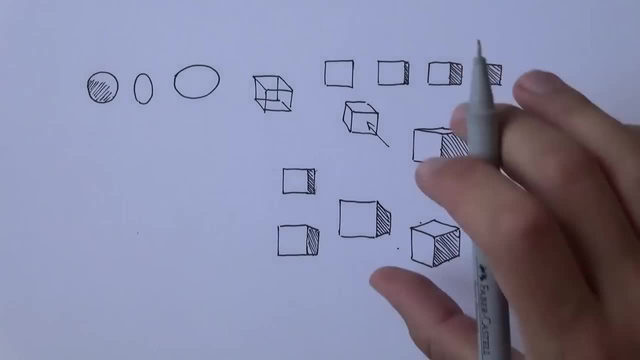 exercise to play around with it. move it around, try and imagine it from different locations, from different angles, and maybe also working with a transparent cube from time to time, so you can kind of turn it around in your head and try and draw it now. you won't always succeed, it's not. 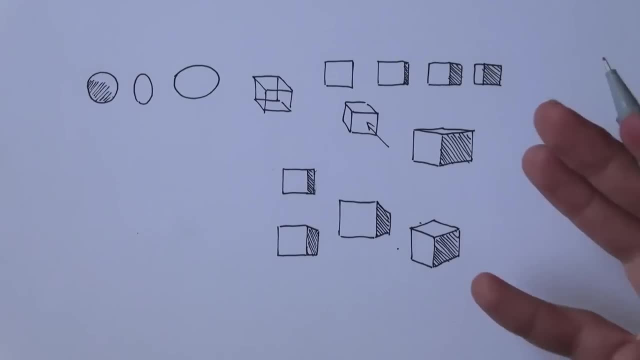 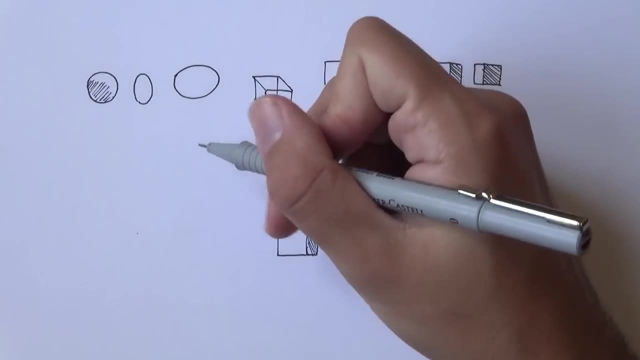 really easy if you don't have that sort of perception, but with practice you'll be able to do that. so this is for the cube. now we have some other shapes. for example, one simple shape is a pyramid. so we can have this sort of a pyramid that has- uh, let's see if i can. 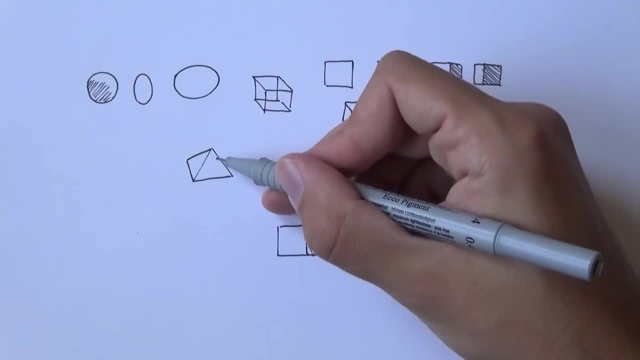 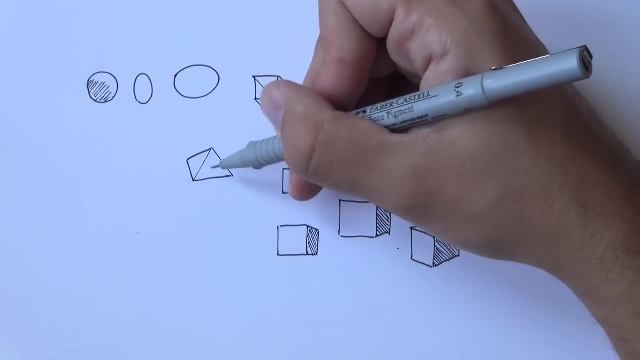 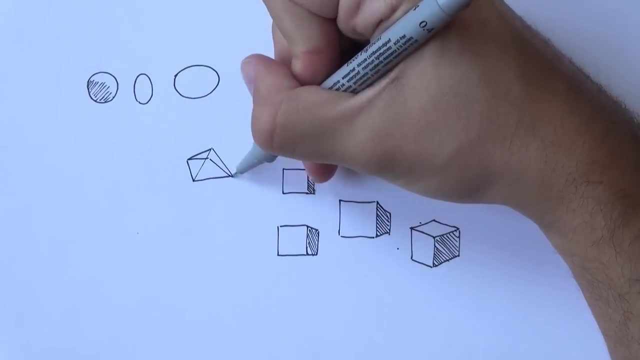 get it to look properly. um, so we have this pyramid, for example. uh, now this pyramid has four sides. it has one meaning: um, four sides on the on the top. okay, i'm gonna show you what i mean in a moment. but there is one, two, and then, if i turn it into a transparent structure, you can see there is one here. 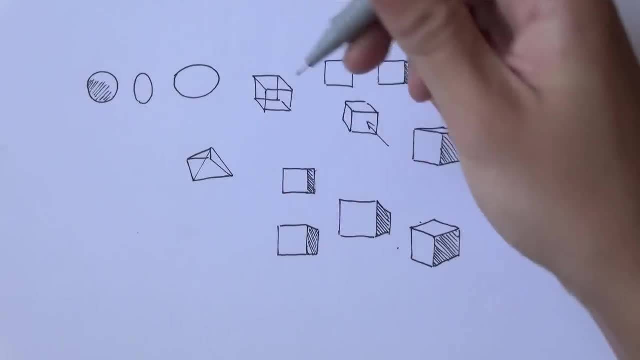 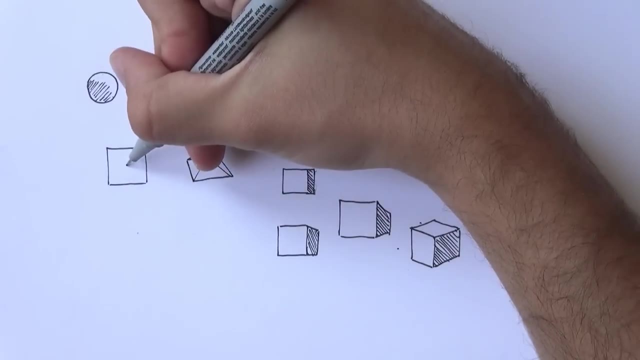 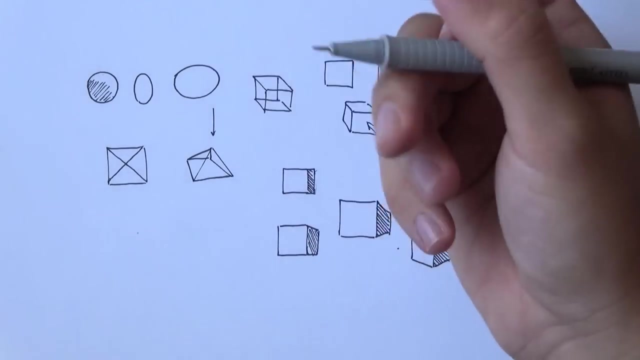 two here, three here and four here. so if we look at it from the very top, we'll get to see something like this: this is the pointy uh center, and we have one and two like this and this is it. so, for example, if uh light would come from this direction, you'll get a sort of heavy shadow. 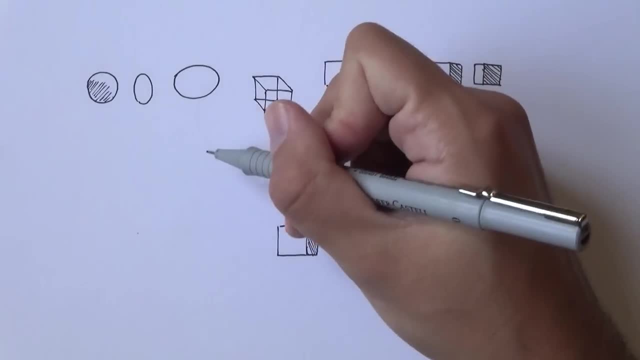 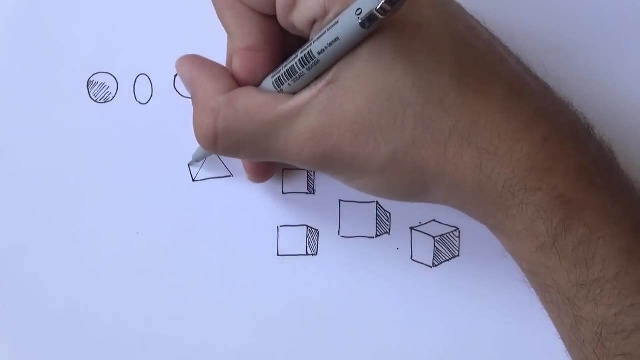 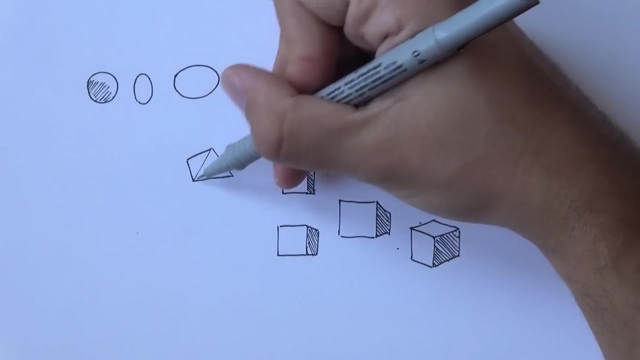 some other shapes. For example, one simple shape is a pyramid. So we can have this sort of a pyramid has- let's see if I can get it to look properly- So we have this pyramid, for example. Now this pyramid has four sides. it has one meaning four sides on the on the top. okay, I'm going to show. 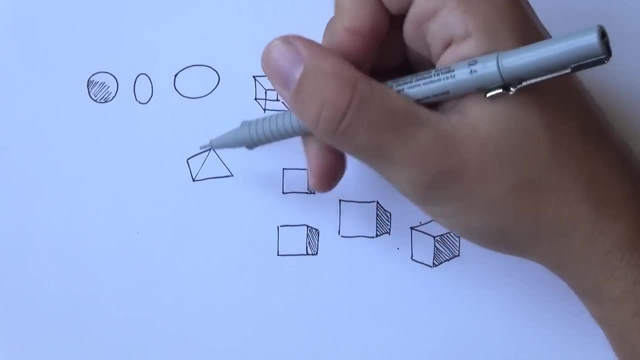 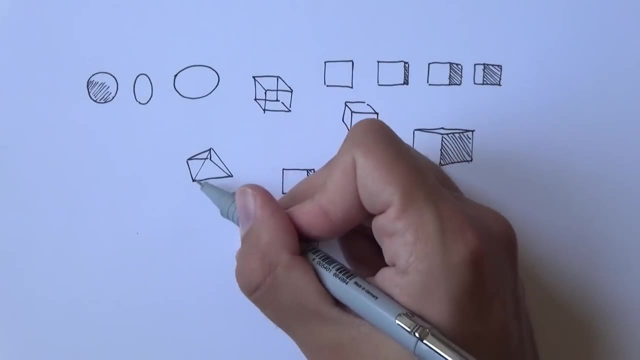 you what I mean in a moment. but there is one, two And then if I turn it into a transparent structure, you can see there is one here, two here, three here and four here. So if we look at it from the very top, 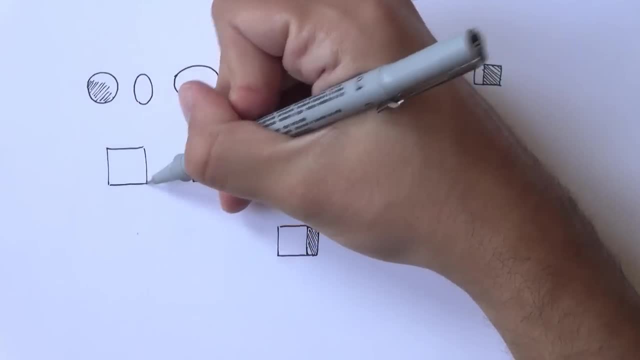 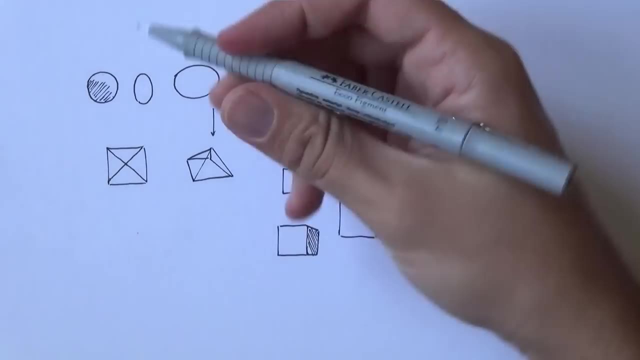 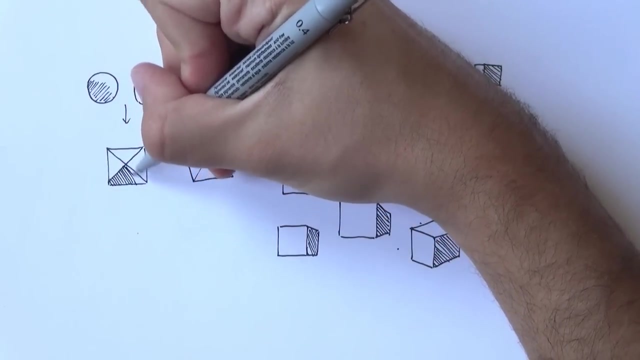 we'll get to see something like this: This is the pointy center, And we have one and two like this, And this is it. So, for example, if light would come from this direction, you'll get a sort of heavy shadow on this side. These ones are going to be a little darker, but not that dark, And you. 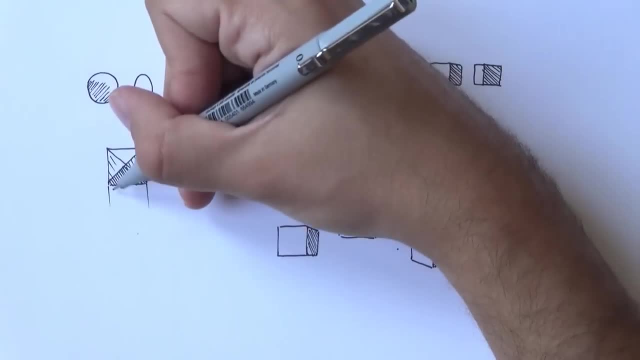 will have a cast shadow, that's sort of the the pyramid casts to this side. Okay, Now, if we move this to the other side, it's going to be a little darker, but not that dark, And you will have a cast shadow, that sort of the the pyramid casts to this side. Okay, Now, if we move this, 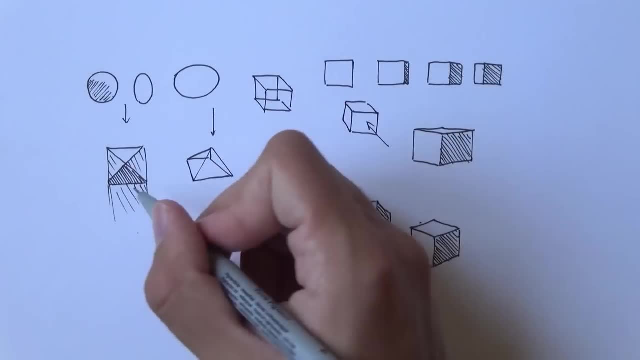 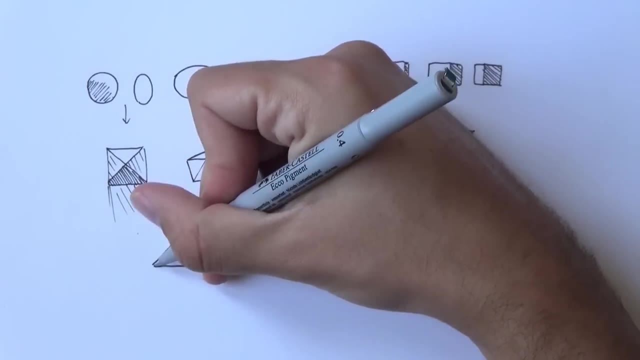 that a bit in space. so let's imagine we're lowering our angle, we're going to get to see more of this side, So I'm just going to draw it a little larger. So more from this side, a little less from this side. So we'll get something like this, And these sides stay kind of. 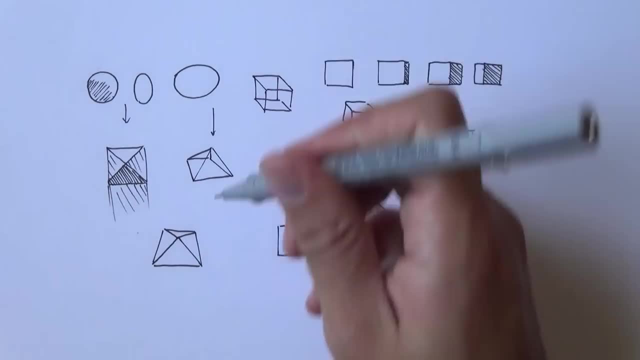 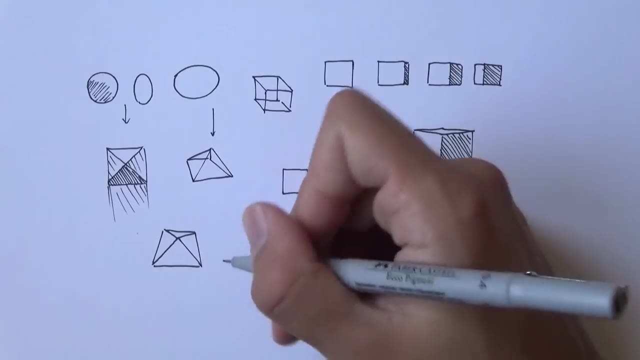 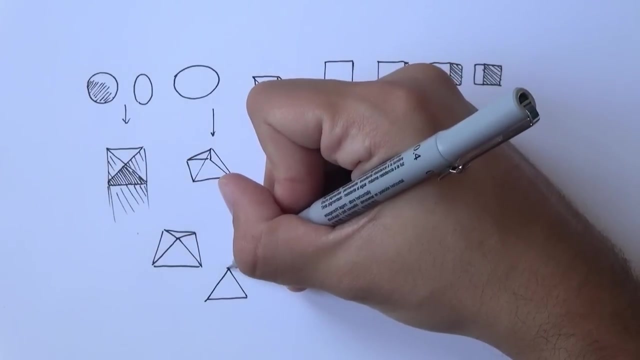 similar And that way you can see it just feels like we went a little lower in space, Okay, But we're still looking at it quite from the top. Now, if we will lower the angle a bit more, we'll get to see even more of this side here, And maybe barely anything from this side and just a bit of the side. 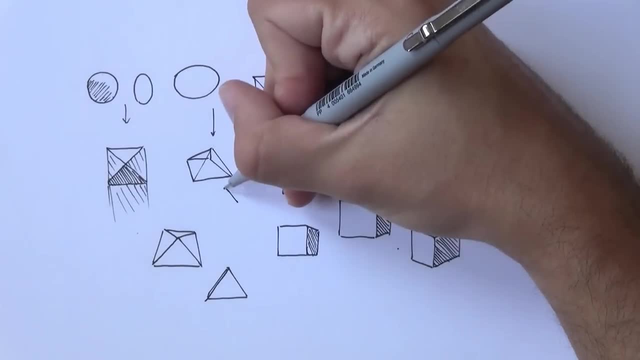 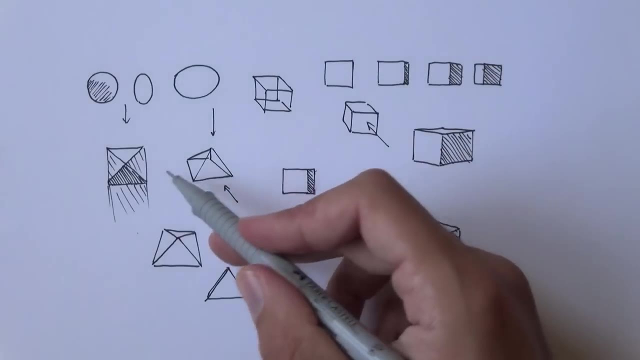 view. So when you get really to a side view, like from here, you'll only see kind of a triangle. Okay, Now, in addition to this pyramid, there's another type of pyramid with three sides. So this, this one is not really I'm not sure if there is any structure that's. 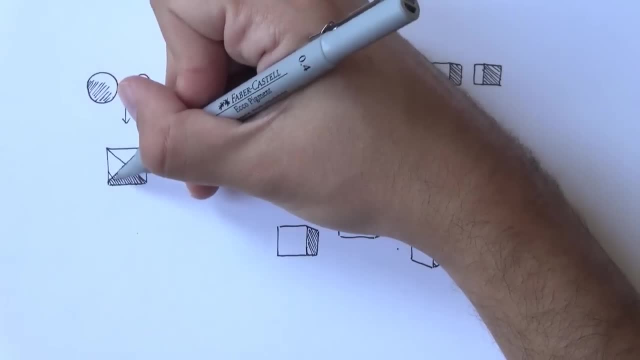 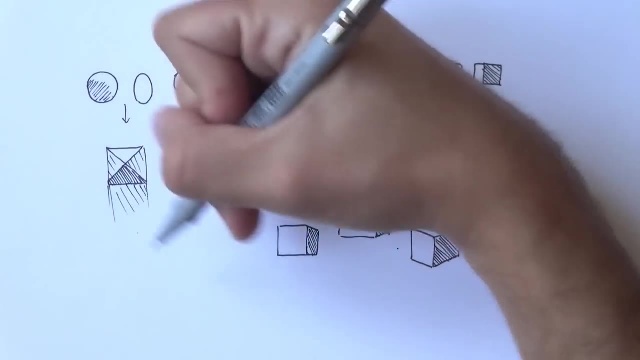 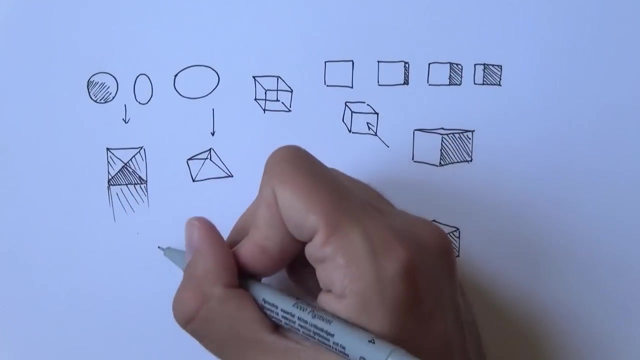 on this side. these ones are going to be a little darker, but not that dark, and you will have a cast, that's sort of the the pyramid casts to this side. okay, now, if we move that a bit in space- so let's imagine we're lowering our angle- we're going to get to see more of this side. so i'm just going to 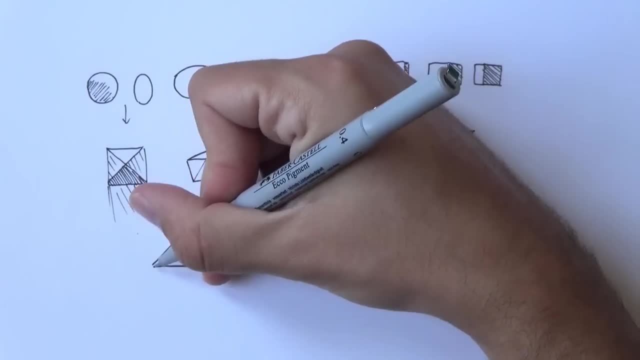 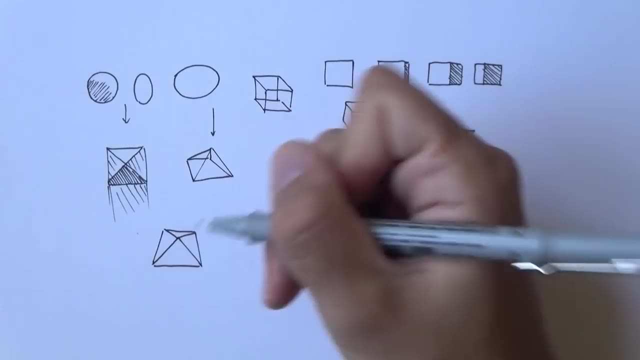 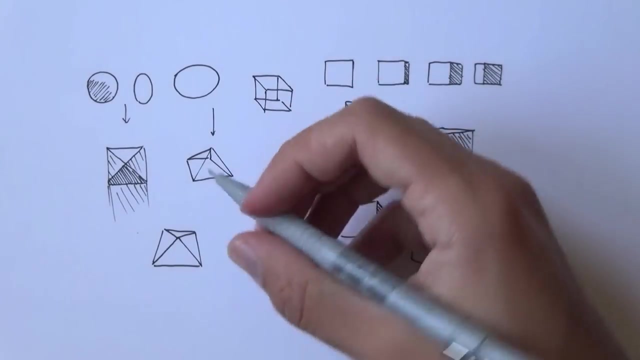 draw it a little larger, so more from this side, a little less from this side, so we'll get something like this, and these sides stay kind of similar, and that way you can see it just feels like we went a little lower in space, okay, um, but we're still looking at it quite from the top. now, if we will lower the angle a bit more, we'll get 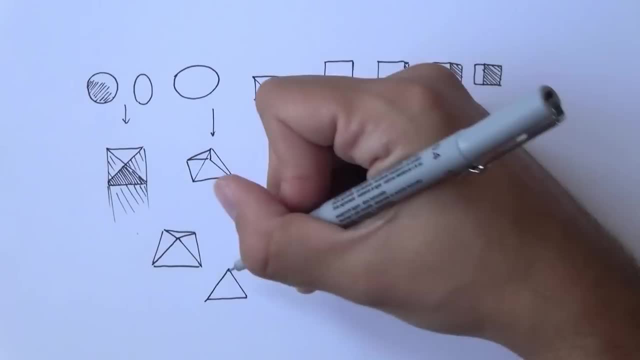 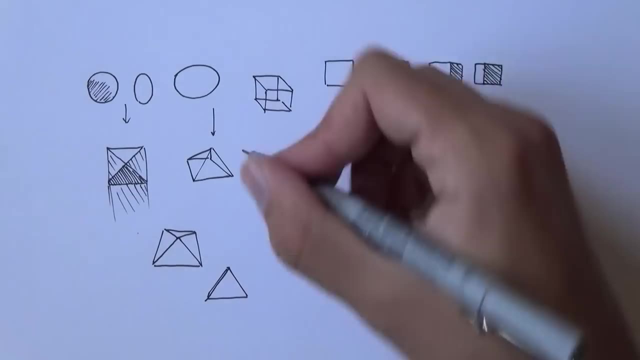 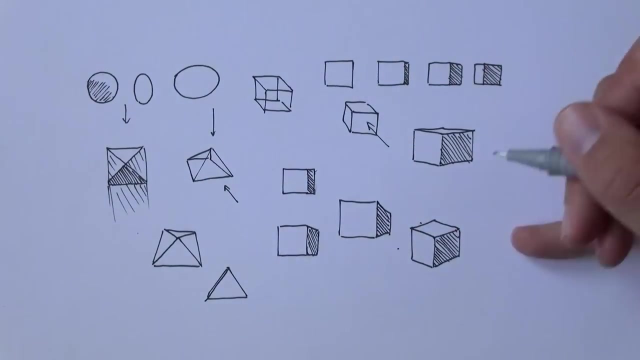 to see even more of this side here and maybe barely anything from this side and just a bit of the side view. so when you get really to a side view, like from here, you'll only see kind of a triangle. okay, now in addition to this pyramid there's another type of pyramid, uh, with three. 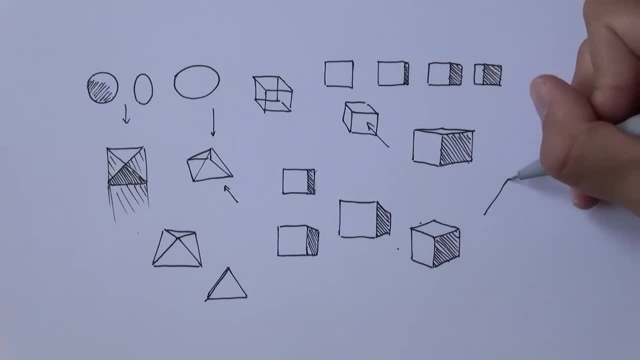 sides. so, uh, this, this one is, uh, not really. i'm not sure if there is any structure that's actually built that way on earth, so let me know in the comment below if you know of one. but anyway, it's this kind of a thing. okay, now the main difference. this is top view. 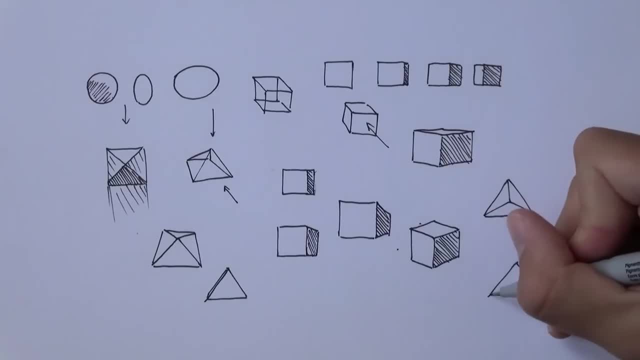 the main difference with this one is that the sides have a different um, there's just less sides- one, two, three- as opposed to one, two, three, four- and so the angle between in the base of the pyramid will be different. so the base here is: maybe this is a. 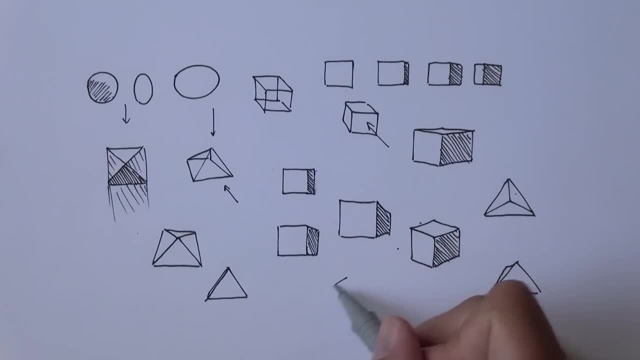 better way to explain it. the base and the perimeter will be different. in this way, i'm going to start with a pyramid and i'll explain it in 2, 2, 5avier before i get to the surface. then, on the arrogant bit, The base is a triangle and then, from the very center, if we sort of raise a line like this, 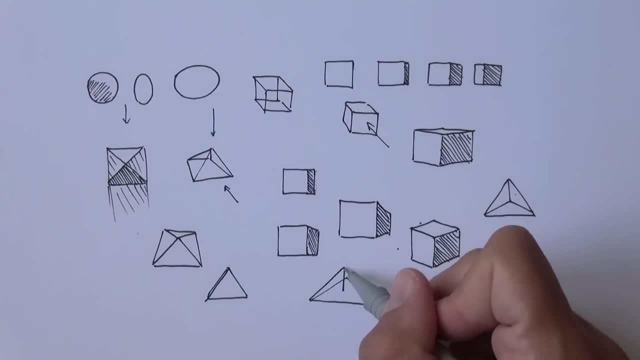 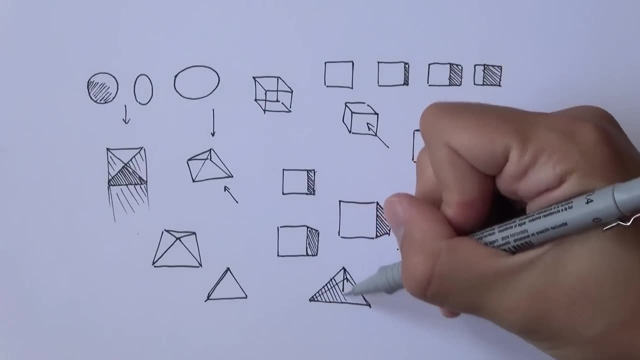 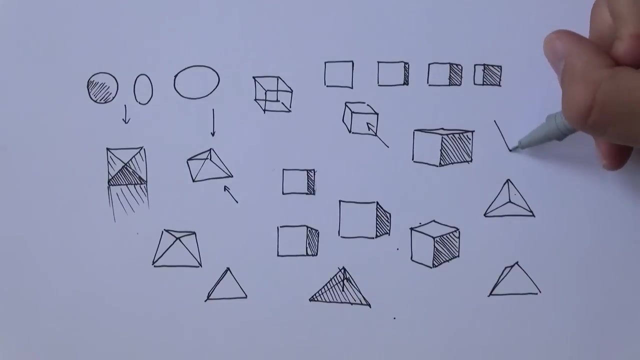 that's perpendicular to the surface and we connect it to the sides, to all of the sides. we're going to get a pyramid, with this being the front wall, the wall that we're facing, Same thing with the square, so we can draw a sort of a like this kind of a shape. 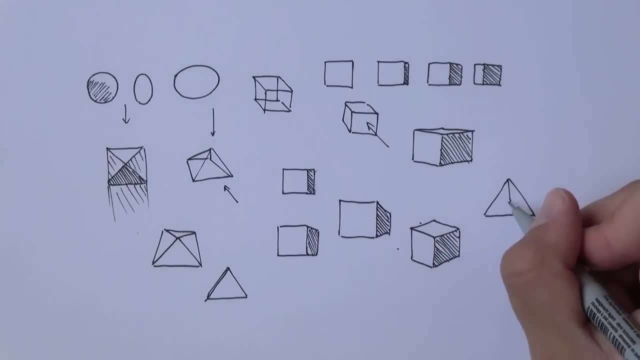 actually built that way on Earth. So let me know in a comment below if you know of one. But anyway, it's this kind of a thing. Okay. Now the main difference- this is top view- The main difference with this one is that the sides have a different, have the. there's just less sides, 123 as opposed. 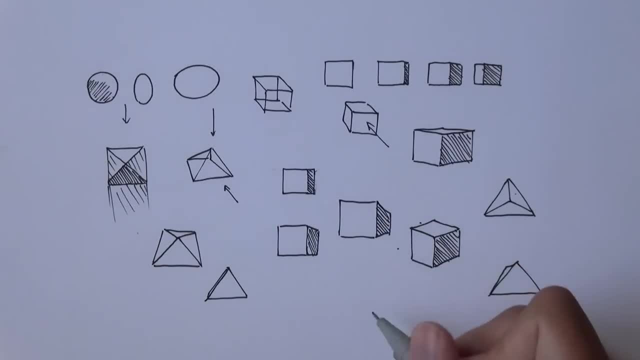 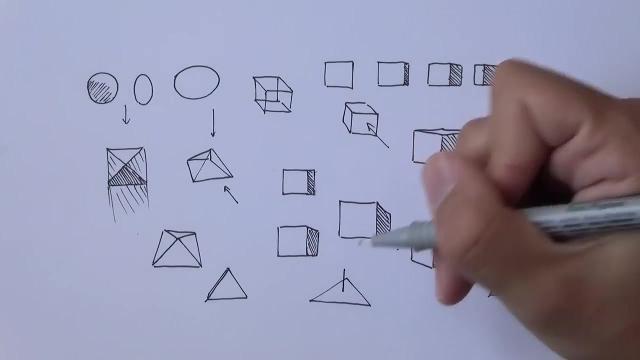 to 1234.. And so the angle between in the base of the pyramid will be different. So the base here is- maybe this is a better way to explain it- The base is a triangle. Okay, And then from the very center, if we sort of raise a line like this, that's perpendicular to the surface. 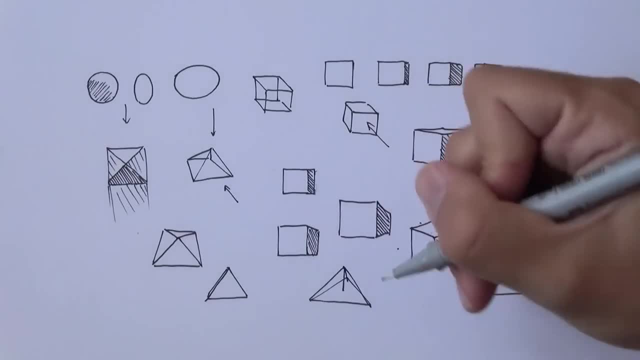 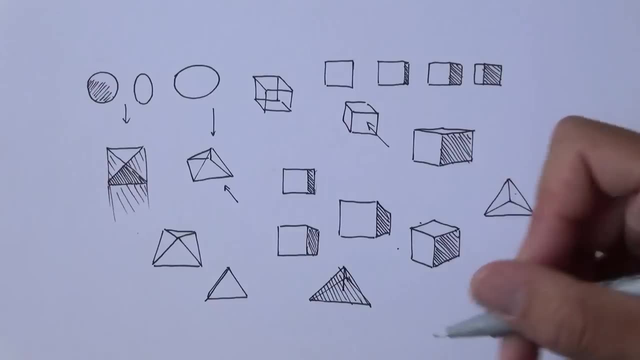 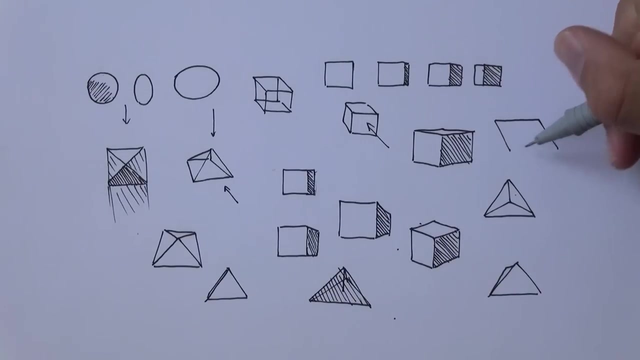 and we connect it to the sides, to all of the sides, we're going to get a pyramid, Okay, with this being the front wall, the wall, that's that we're facing Same thing with the square. So we can draw a sort of a like, this kind of a shape. And if we find the center and the center, 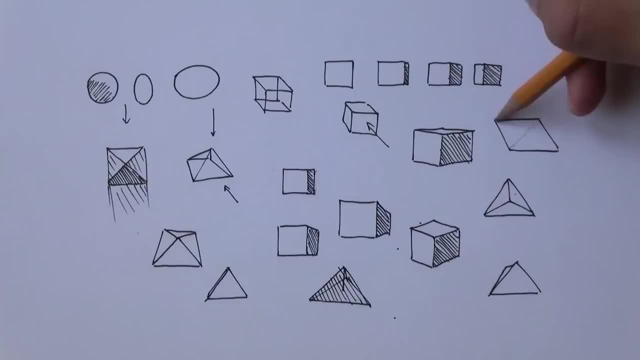 can be found in the center, So we can find the center, and the center can be found in the middle, So we can find the center, and the center can be found very easily, by the way, by just connecting these two. okay, like this, we're gonna point, just put a dot in there. 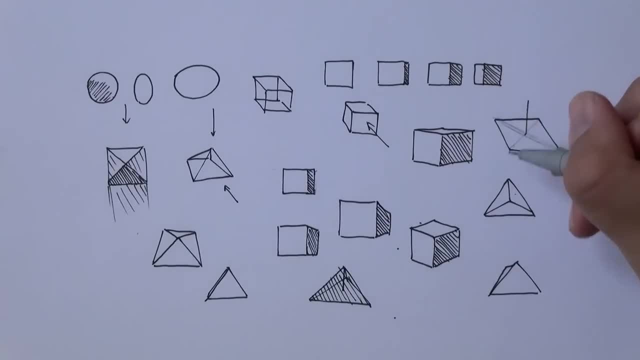 raise it up, okay, using an imaginary line and then connected to all sides of the cube And you can see my lines are wobbly. that's perfectly fine. So the main difference is in the angles here. here we have a 90 degree angle And here we have a smaller angle. Okay, 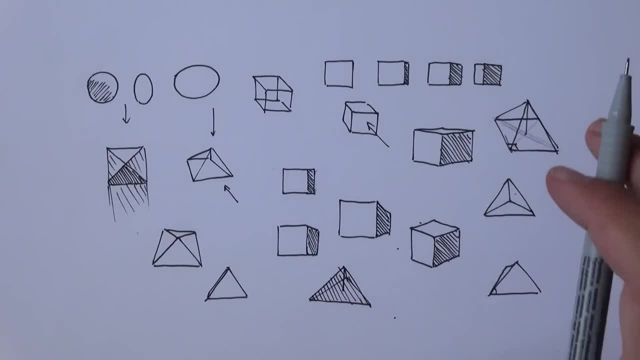 that's the main difference. So hopefully all of this makes sense. Now I'm going to rearrange the paper a bit. Now I'm going to rearrange the paper a bit. Now I'm going to rearrange the paper a bit. 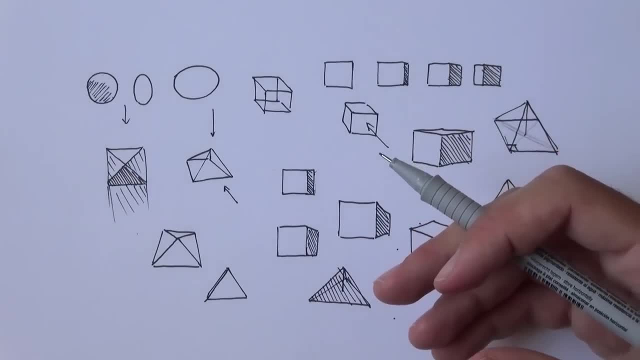 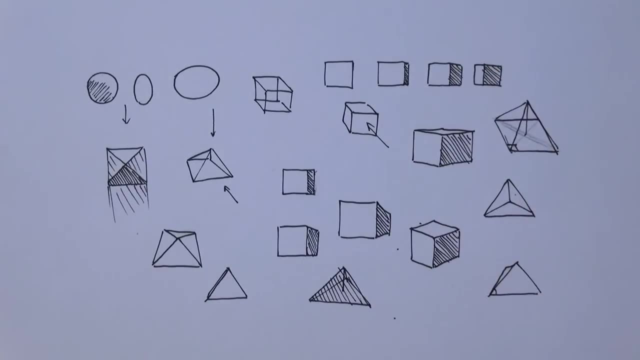 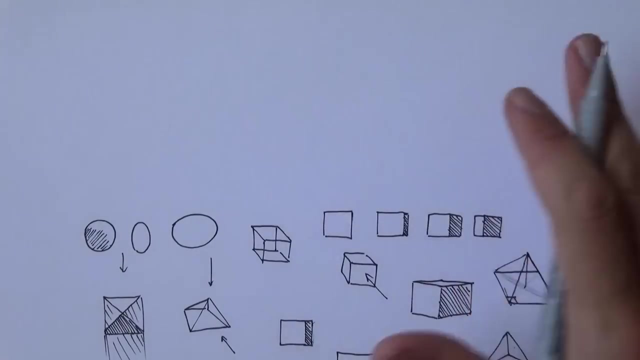 And I want to show you my sort of my, my take on this exercise and how you can apply it, because maybe some of you can already do all of that, Okay, Okay. so the thing I'm going to demonstrate to you now. funny enough, I started doing as a kid- Okay, I loved doodling these kinds of shapes. 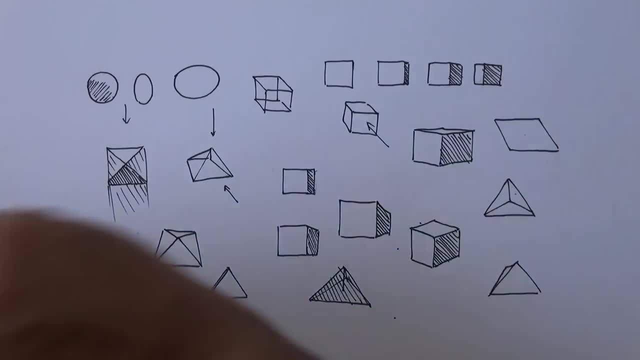 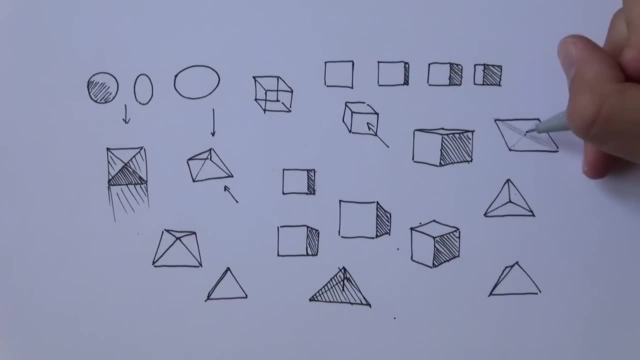 and if we find the center- and the center can be found very easily, by the way, by just connecting these two like this we're going to point- just put a dot in there, raise it up using an imaginary line. 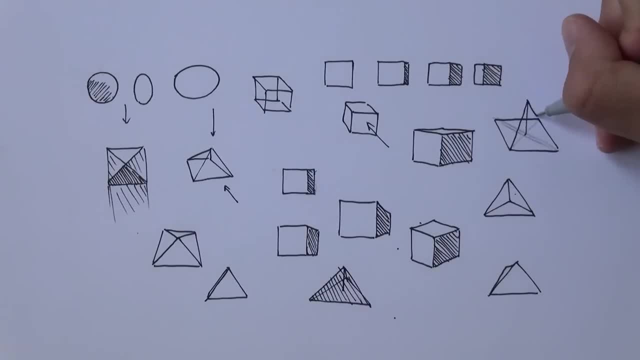 and then connect it to all sides of the cube And you can see my lines are wobbly. That's perfectly fine. So the main difference is in the angles here. Here we have a 90 degree angle and here we have a smaller angle. 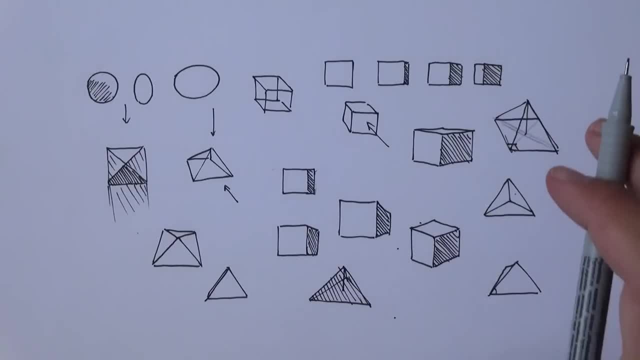 Okay, that's the main difference, So hopefully all of this makes sense. Now I'm going to rearrange the paper a bit and I want to show you my sort of my take on this exercise and how you can apply it, because maybe some of you can already do all of that. 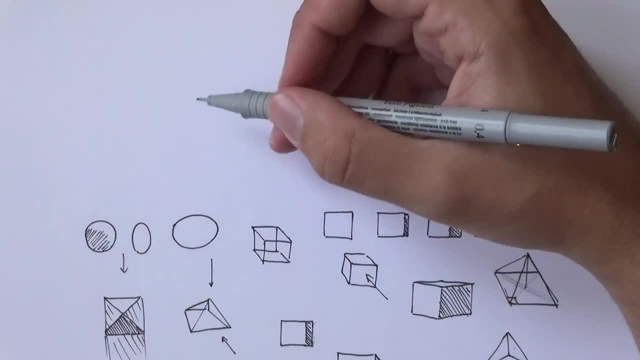 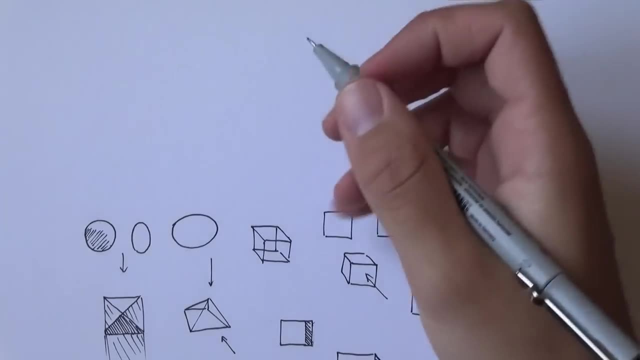 Okay, so the thing I'm going to demonstrate to you now. funny enough, I started doing as a kid. Okay, I loved doodling these kinds of shapes. when I was younger Now, what I used to do is create imaginary three-dimensional shapes. 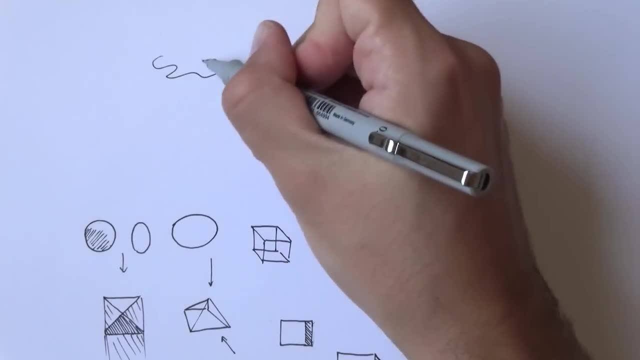 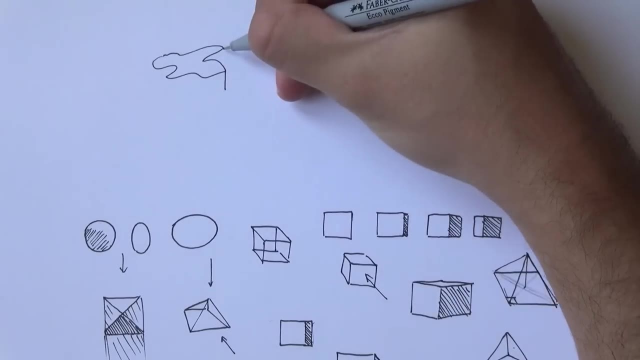 And what do I mean by that? I would just make a very weird sort of scribbly shape, and then I'll imagine I'm giving it three-dimensionality. So what I would do is just drop some lines like this and kind of connect them using a line that follows: 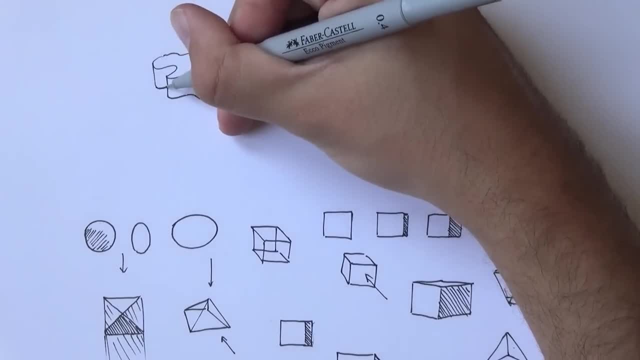 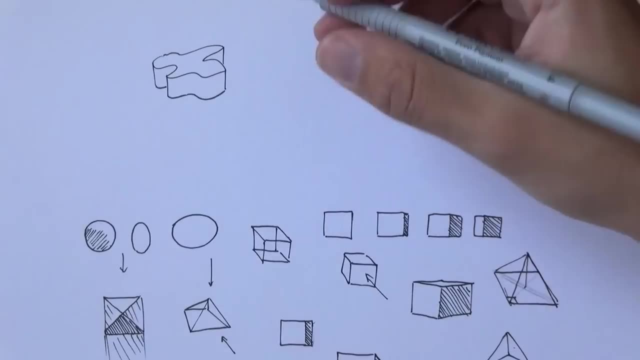 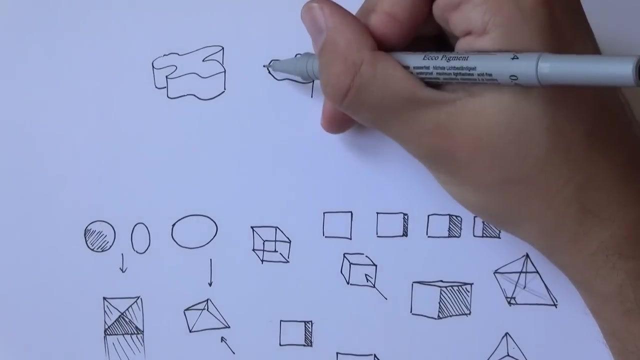 adheres to the previous line, I put Okay, And that way you get a very random three-dimensional shape And I used to do this one all the time And this is really good practice because it trains you in your eyes and your hand to follow the shape you already did. 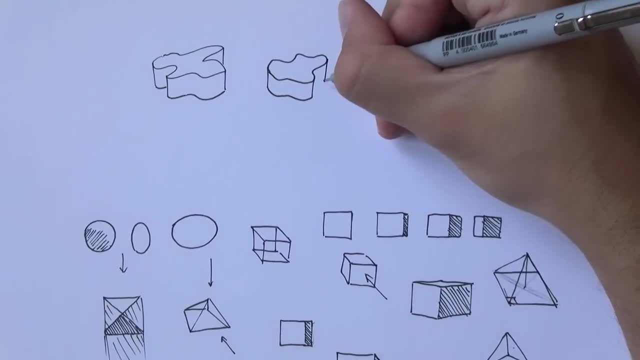 and sort of give it a bit of a height. Now, why is this great? Because a very common mistake I see with beginners is, for example, if you want to draw a cylinder shape like sort of a soda can, So what you will get is 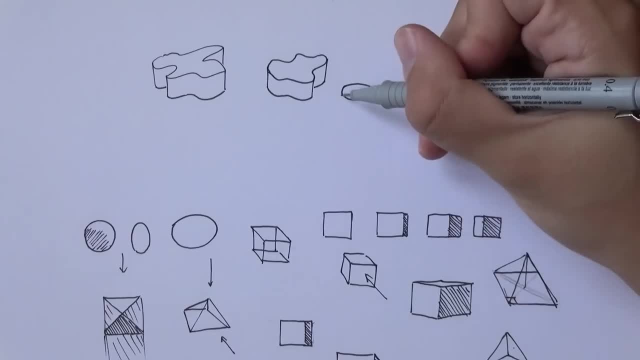 A lot of people do this. They draw the top part like that, Then they draw the sides and then the bottom is like this, And this is not the way it should be. This area should follow the structure of this. Unless the shape is, when looked at from the side will look kind of like. 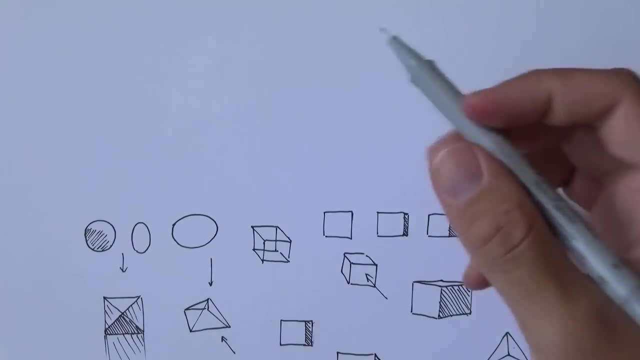 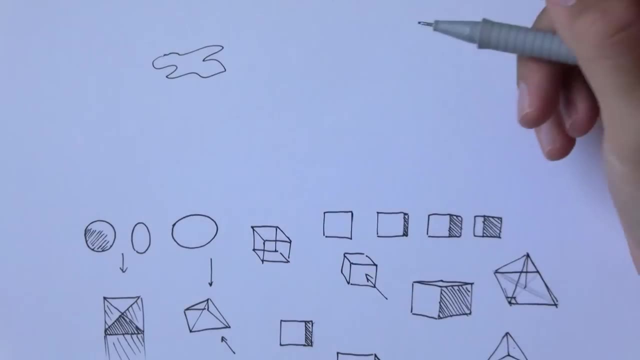 when I was younger. Now, what I used to do is create imaginary three dimensional shapes. And what do I mean by that? I would just make a very weird sort of scribbling shape, And then I'll imagine I'm giving it three dimensionality. So what I would do? 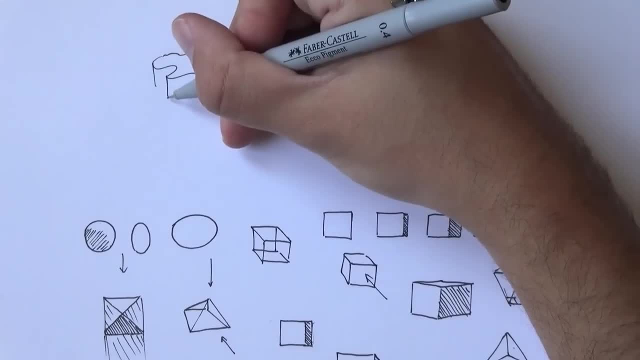 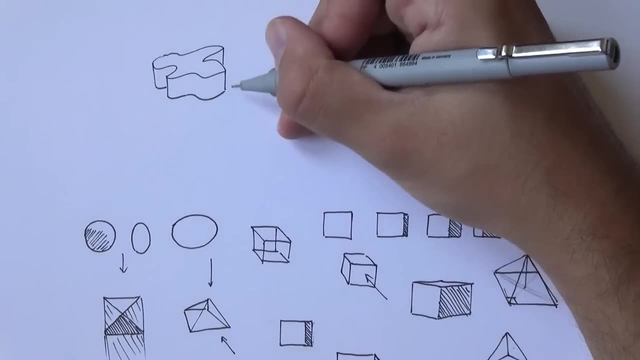 is just drop some lines like this and kind of connect them using the line that follows adheres to the previous line. I put okay, And that way you get a very random three dimensional shape, And I used to do this one all the time And this is really good practice. 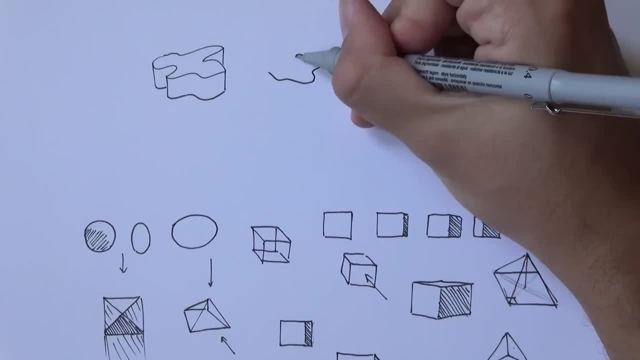 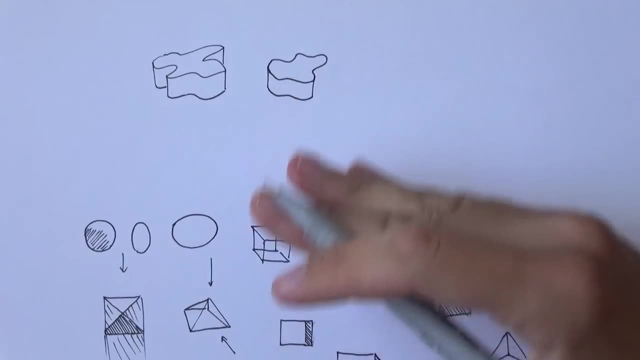 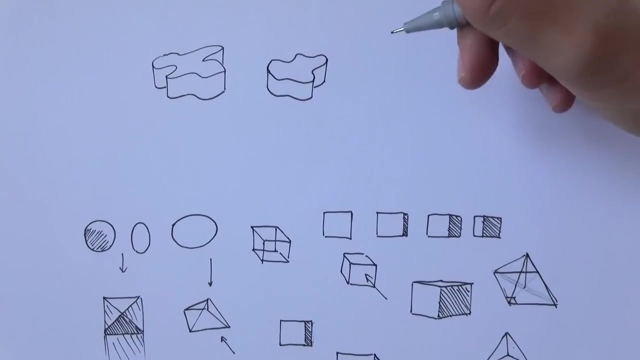 because it's trains you in your eyes and your hand to follow the shape you already did and sort of give it a bit of a height. Now why is this great? because a very common mistake I see with beginners is, for example, if you want to draw a cylinder shape like like sort of a soda, soda can. 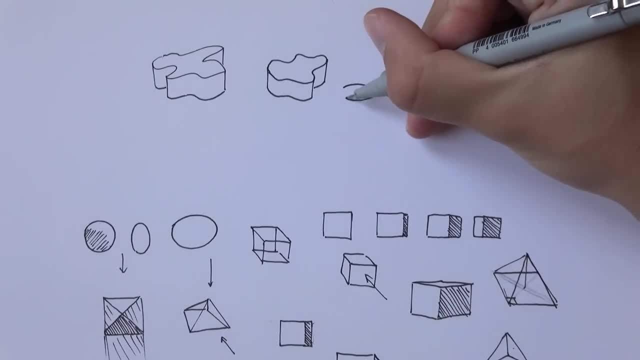 So what you will get is a lot of people do this. they draw the top part like that, Then they draw the sides and then the bottom is like this, And this is not the way it should be. this area should follow the structure of this, unless the shape is. 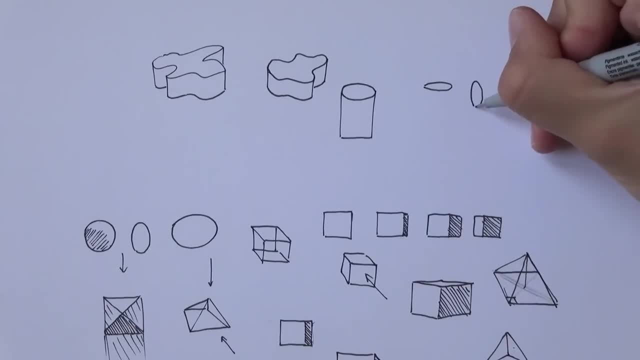 at from the side will look kind of like. it's really hard to do that, But I'll try. like this: Okay, this is what this would look like from the side. Okay, maybe from sort of three quarters it will look something like this: Okay, but nothing really looks like this. 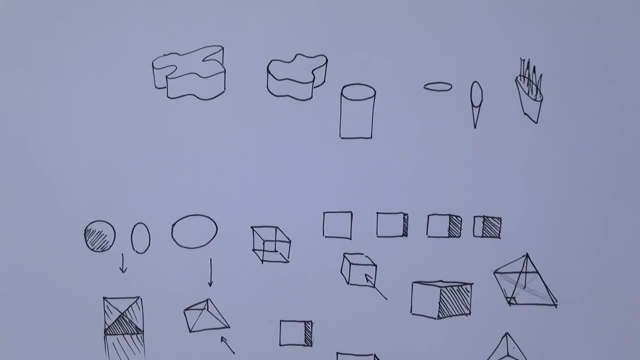 except for the french fries kind of packaging. you know, usually if you draw like a soda can or something like this, it's just going to be a circle, two lines for the sides and another circle. Okay, now, if you remember, I showed you a bit of perspective here, So we can put this one in. 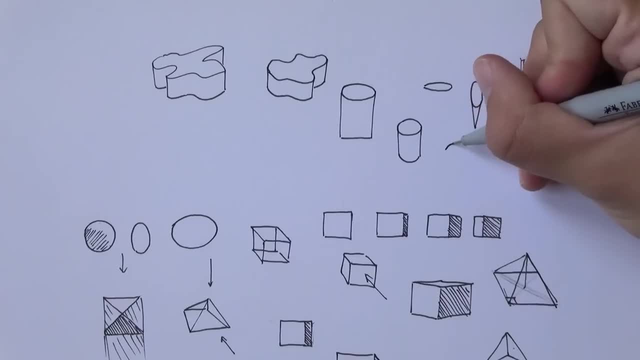 perspective too. So what? the way to do this is just by drawing a circle. then the lines for the sides go a bit inwards, like that, Okay. And then you add this rounded top of the part of the bottom, Okay. Now, again, this happens when our distance, our point of view to this area is significantly 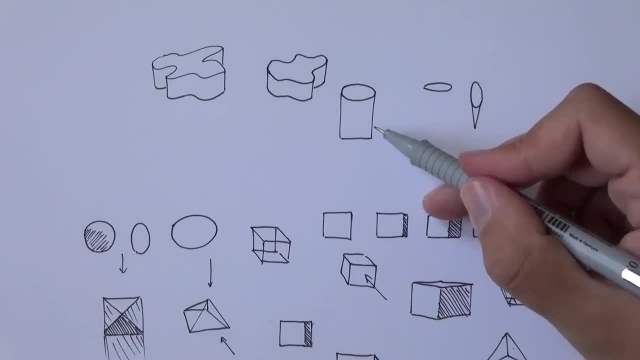 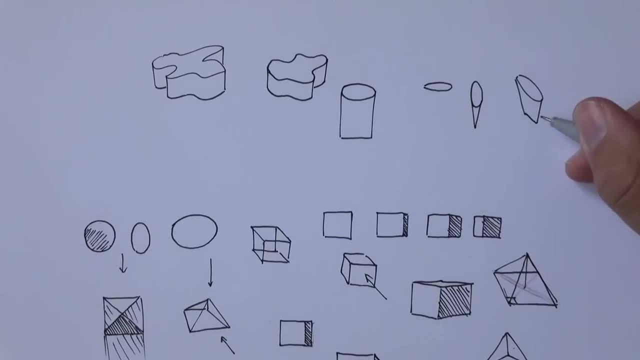 It's really hard to do that, but I'll try, Like this: Okay, this is what this would look like from the side. Okay, Maybe from sort of three-quarters it will look something like this: Okay, But nothing really looks like this. 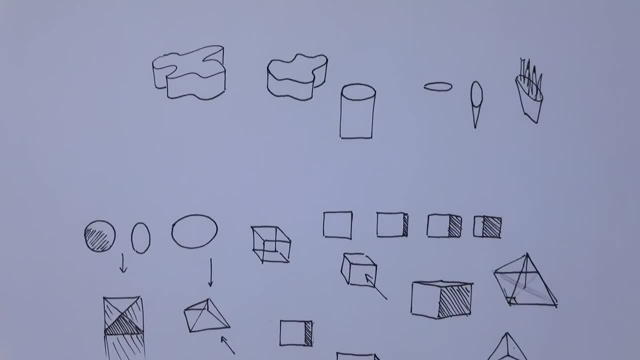 Except for the french fries kind of packaging. you know, Usually if you draw like a soda can or something like this, it's just going to be a circle: two lines for the sides and another circle. Okay, Now, if you remember, I showed you a bit of perspective here. 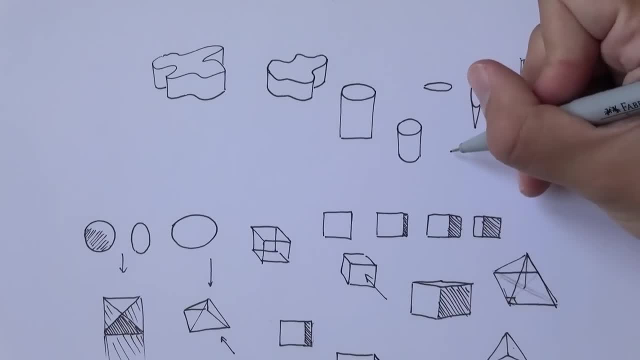 So we can put this one in perspective too. So the way to do this is just by drawing a circle, Then the lines for the sides go a bit inwards, like that, Okay, And then you add this roundness, And then you add the top part at the bottom. 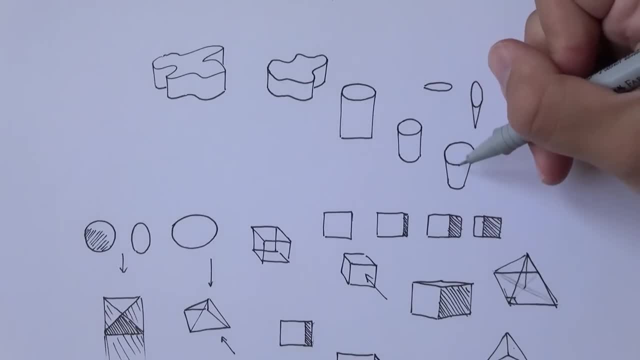 Okay, Now again, this happens when our distance, our point of view to this area is significantly different from this area. So you usually won't see. You will see it a bit with soda cans if you hold them close to your eyes. 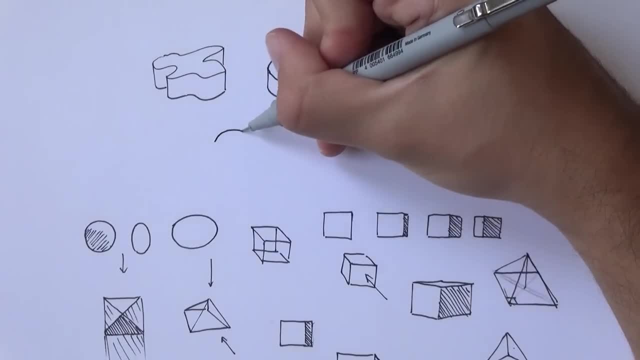 But where you will see this is sometimes you may see like a construction works And then you'll have this sort of open pipes lying around somewhere And you may see them sort of moving in perspective. Okay, If you look at it more at the front, this is interesting. 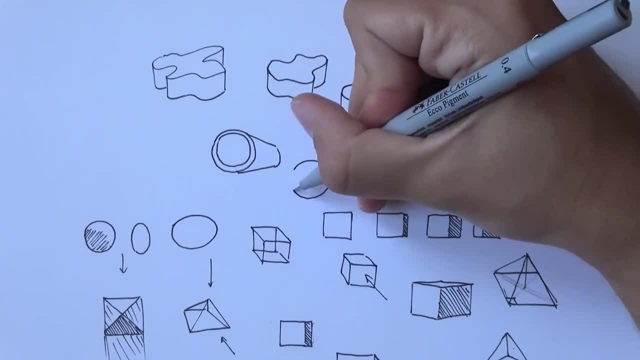 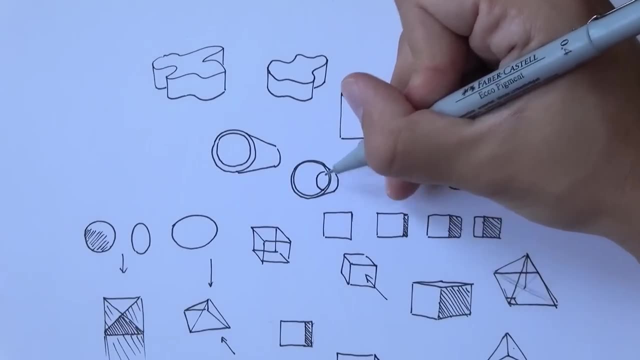 So let's imagine there's a hole on both sides. So if you look at it a bit more kind of from the front, you'll even get to see the opening on the other side. Okay, So this is sort of like a tunnel that you can go through, almost. 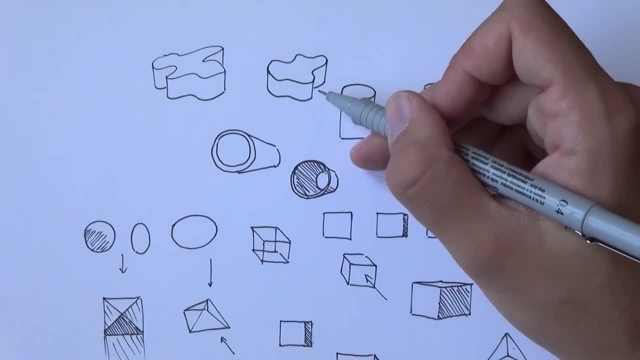 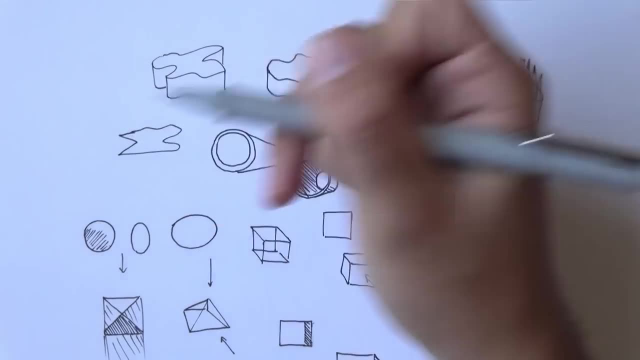 Now I just want to add one more touch to this sort of exercise. You can add shading to that. Okay, Do sort of your scribbly kind of shape and just try getting it to be three-dimensional, And then you can just add a random light source. 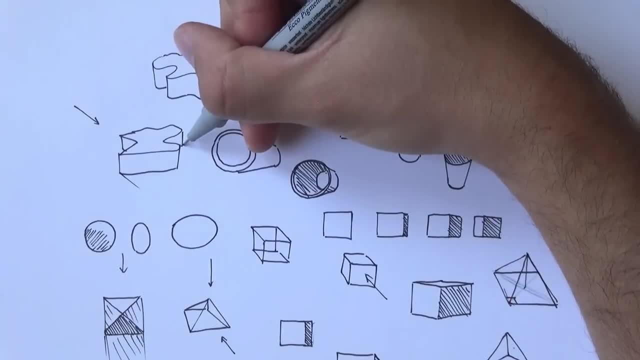 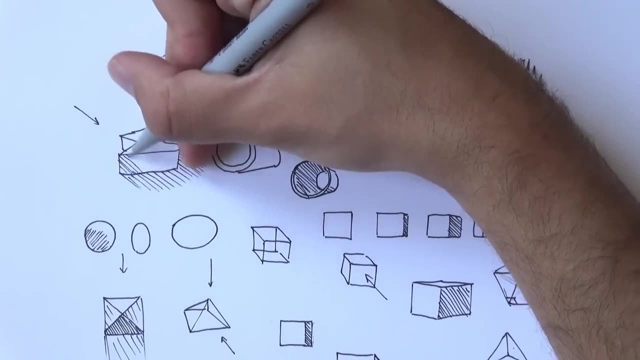 So, for example, light comes from here And you can kind of just draw this shadow, cast shadow or maybe shadow on the object itself, And you can kind of imagine what areas are going to be in the shadow, what areas are going to be more well lit. 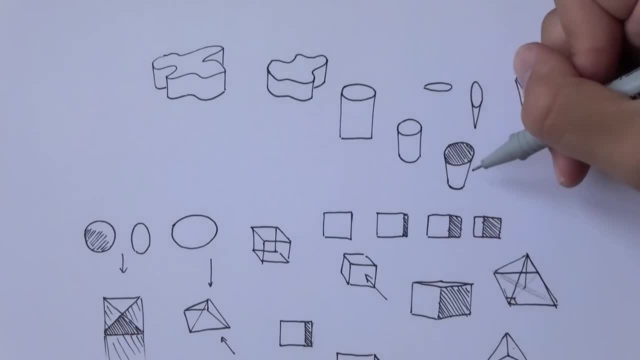 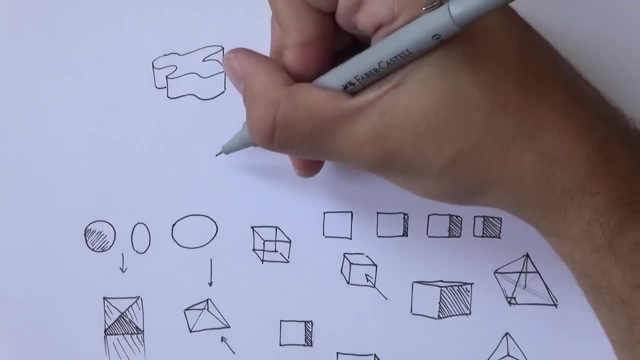 different from this area. So you usually won't see what you will see. you won't see a lot of this. You will see it a bit with with soda cans if you hold them close to your, to your eyes. But where you will see this is sometimes you may see like construction works And then you'll have this. 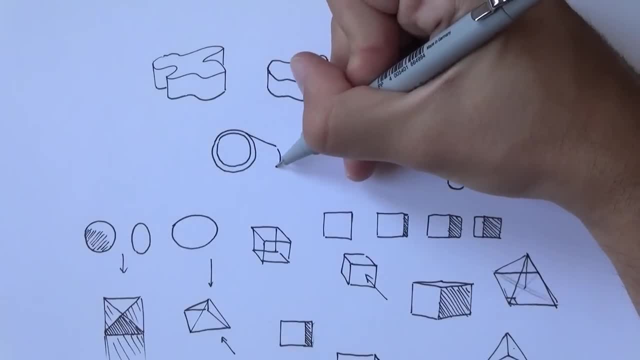 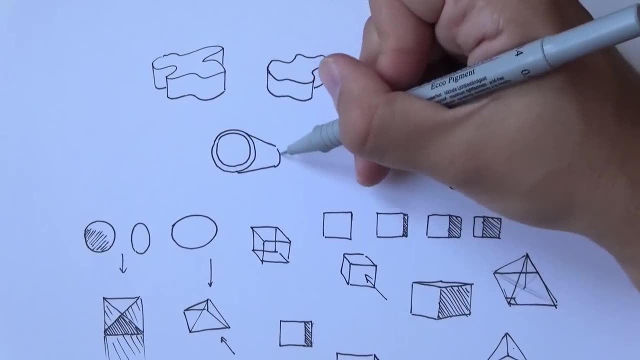 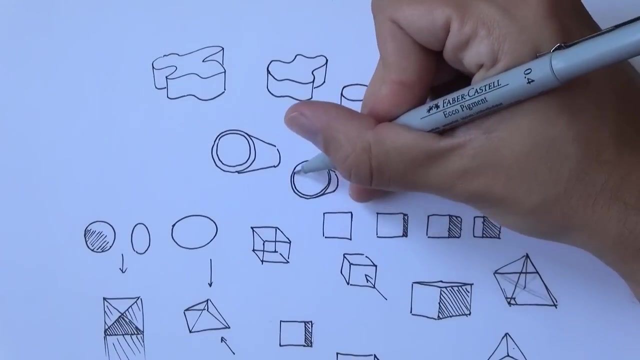 sort of open pipes lying around somewhere and you may see them sort of moving in perspective. Okay, If you look at it more at the front, this is interesting. So let's imagine there's a hole on both sides. So if you look at it a bit more kind of from the front, you'll even get to see. 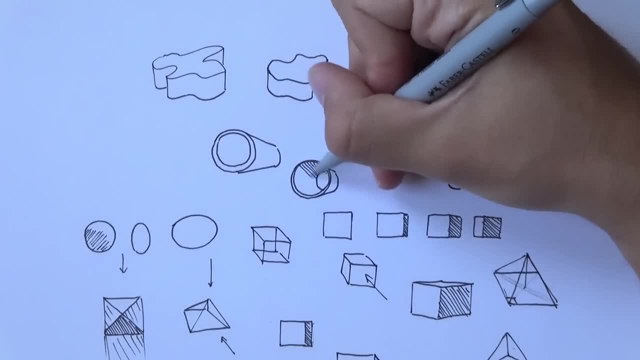 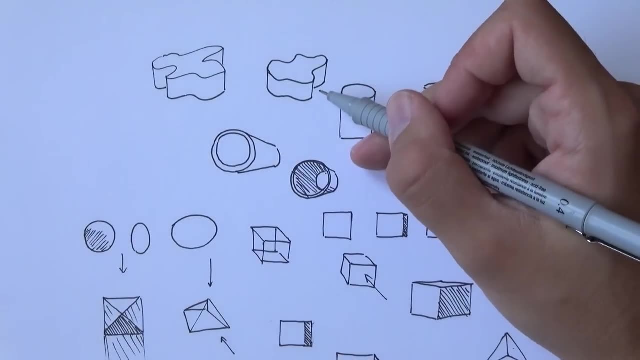 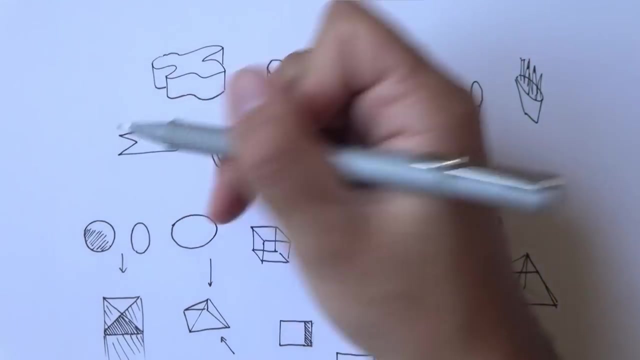 opening on the other side, Okay, So this sort of like a tunnel that you can go through almost now. And I just want to add one more touch to this sort of exercise And you can add shading to that. Okay, so you can do sort of your scribbly kind of shape And just try getting it to be. 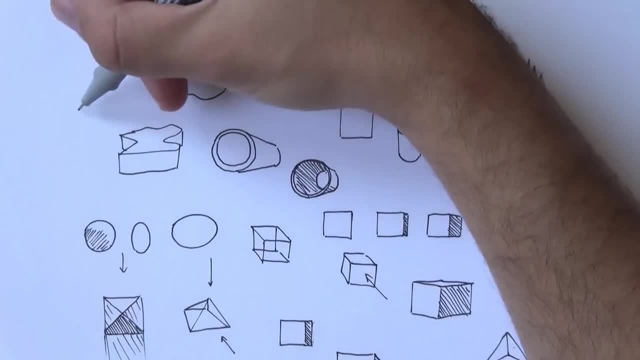 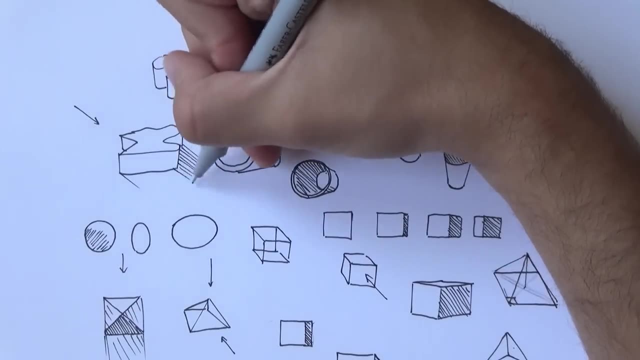 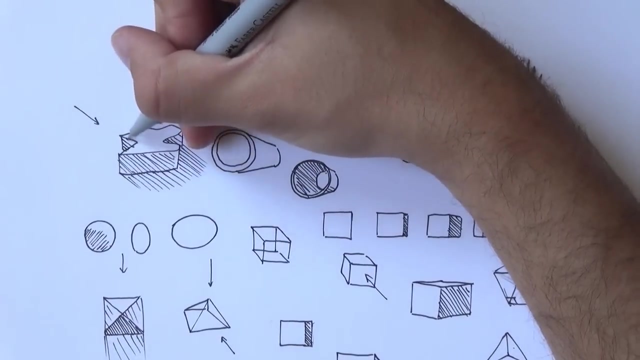 three dimensional, And then you can just add a random light source. So, for example, light comes from here And you can kind of just draw this shadow, cast shadow, or maybe shadow on the object itself, And you can kind of imagine what areas are going to be in the shadow, what areas are going to be more well lit, And this is just 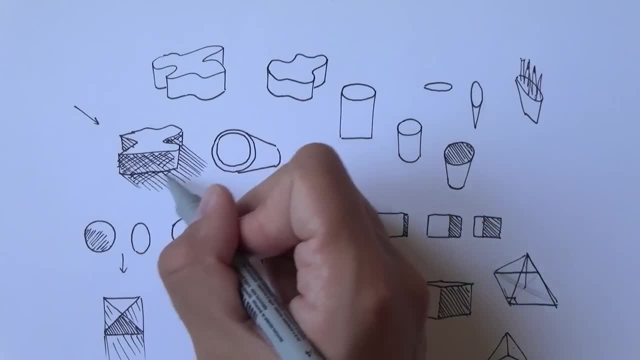 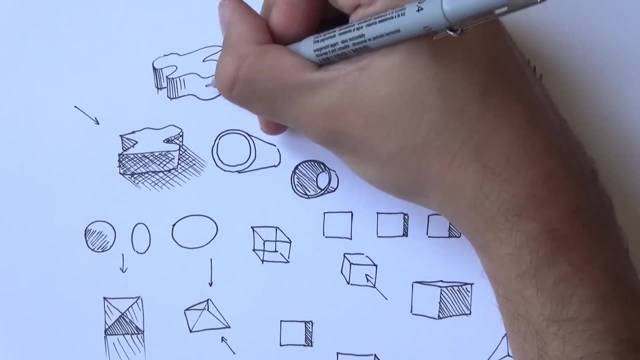 a really fun exercise. You can do this also with kind of artificial lighting, So, for example, just add a bit of shadows like this, And this really trains your ability to kind of hatch and do these kinds of lines: 007, 008, 009. 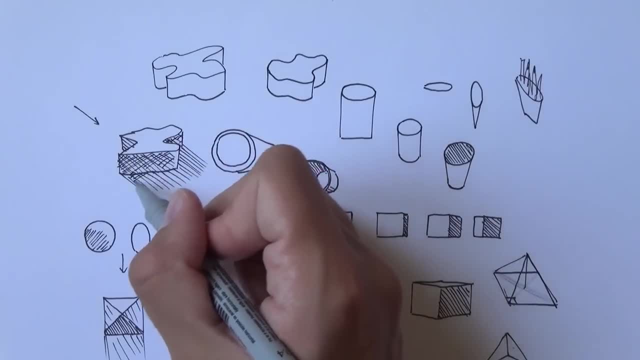 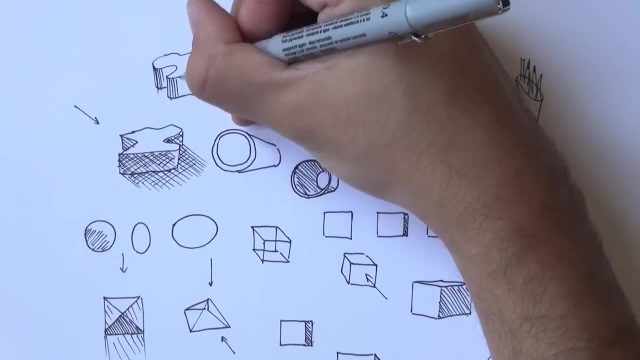 And this is just a really fun exercise. You can do this also with kind of artificial lighting. So, for example, just add a bit of shadows like this, And this really trains your ability to kind of hatch and do these kinds of lines. 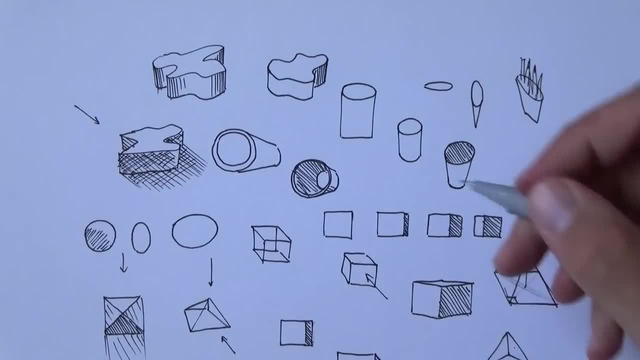 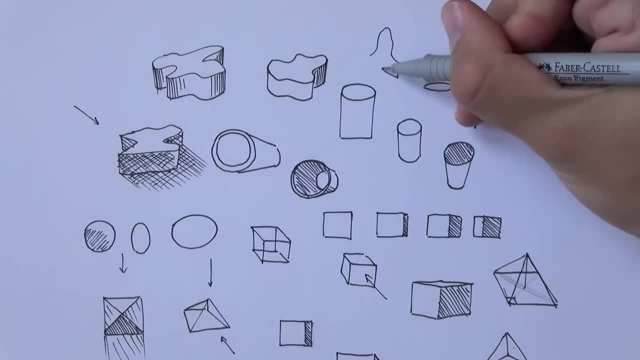 It's just a very fun thing to do when you doodle or when you just kind of sketch for fun. This is an exercise I used to do when I was really young and it's just very fun. You can rotate the angles so you can work to the sides. 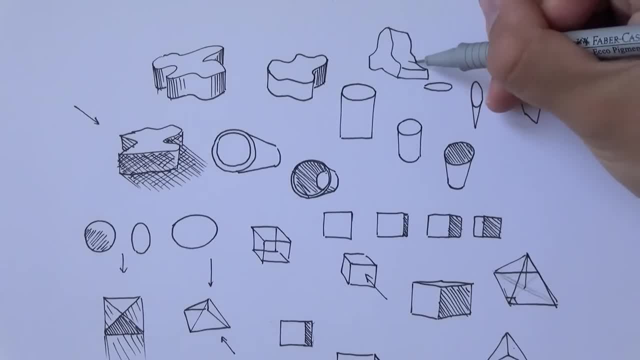 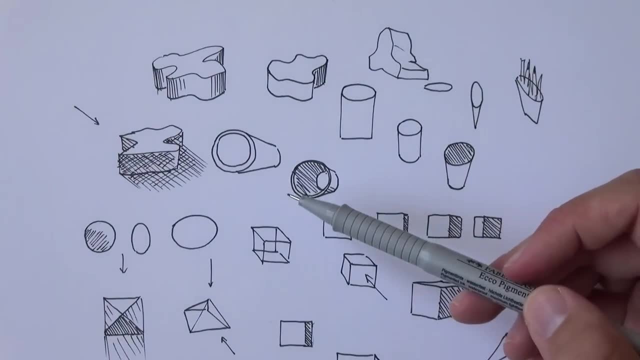 You can also skew the shape a bit So that it actually has a bit of weirdness element to it. This is really all just experimentation. Doing this a lot and on a regular basis will really improve your abilities to sketch and to draw what you see. 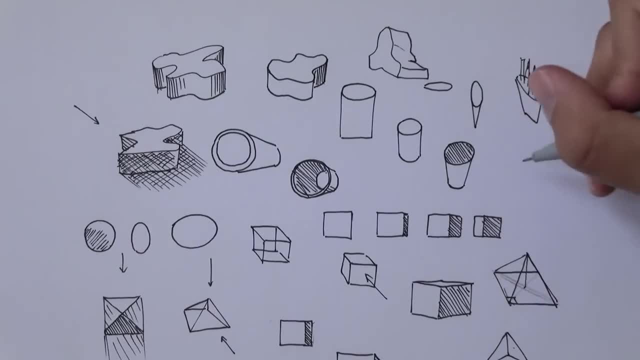 Because, again, the basis for buildings is this: It's the cube. So if I see a building and I want to sort of draw it, or even as a preparation for watercolor painting, that's basically sort of a cube: a cube, elongated cube and with windows. 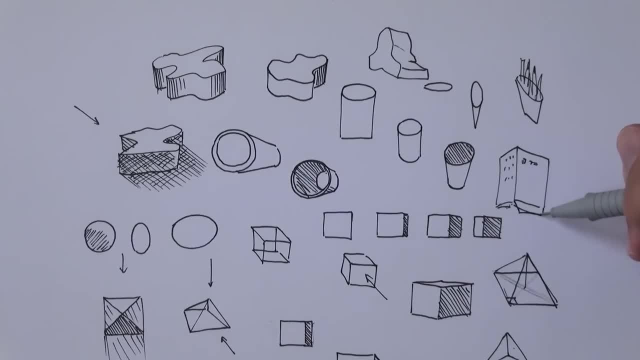 With some more details you can see here. Maybe there's an awning here, maybe there's a restaurant at the bottom, but the concept stays the same. It's just this sort of a building. there's an antenna, whatever it is. 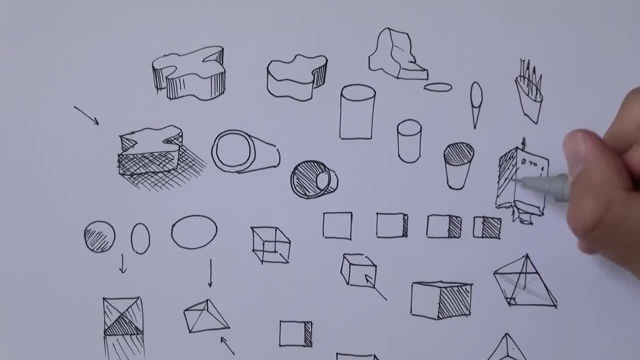 And it's just so simple once you get the sort of basic shapes to it. okay Now, I went through a lot in this video, so what I'm curious to know is, if there's anything you want me to dive even deeper, I want you to let me know. okay. 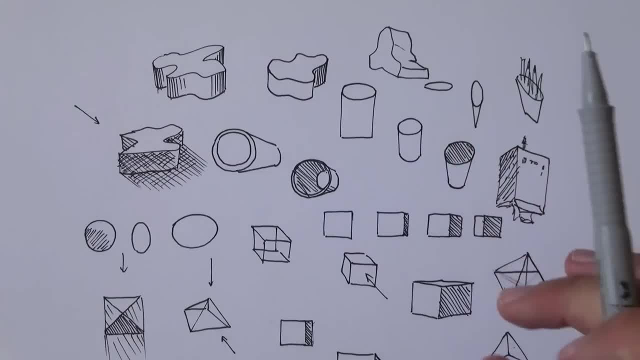 Maybe you want us to sort of analyze the cube on many different angles and just zoom in on that. maybe the pyramids, maybe this weird sort of exercise, maybe the shading part. Let me know in a comment below if you want to know more about any of these specifics. okay, 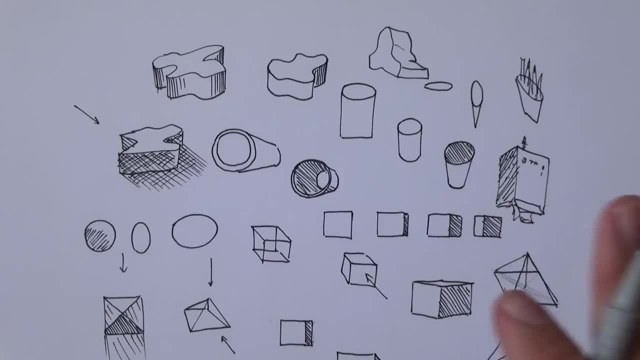 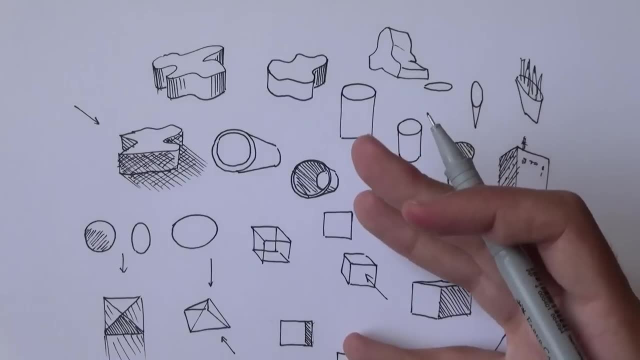 I kind of dumped a lot of things at you. so you just, if you want something specific or something in particular, if you want us to dive into any concept that has to do with three-dimensional shapes, let me know in a comment below. okay, 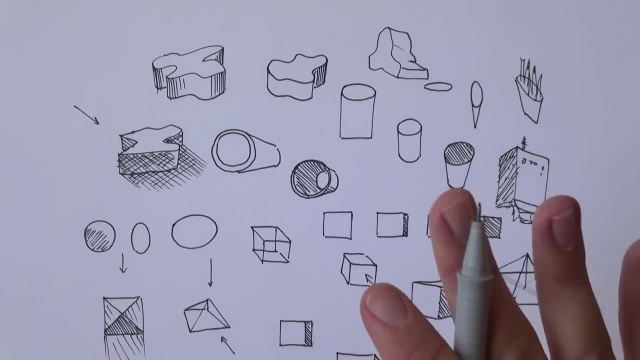 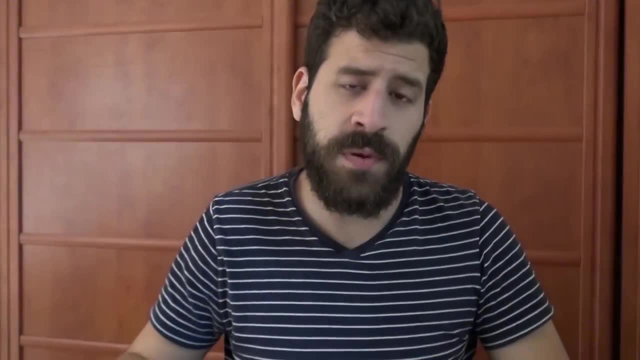 I really hope you enjoyed this demo. Let's change the angle and wrap up the video. Okay, friends, here are all of our little doodles here. I hope you enjoyed this video and again, as you saw, I went through quite a bit of things here. 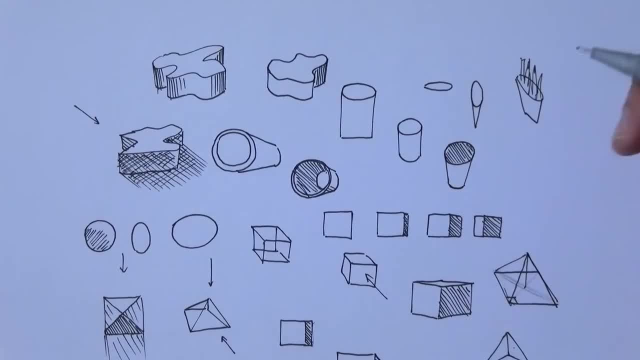 very fun thing to do when you doodle or when you just kind of sketch for fun. This is an exercise I used to do when I was really young and it's just very fun. You can rotate the angles so you can work to the sides. You can also skew the shape a bit so that it actually has a bit of weirdness element. 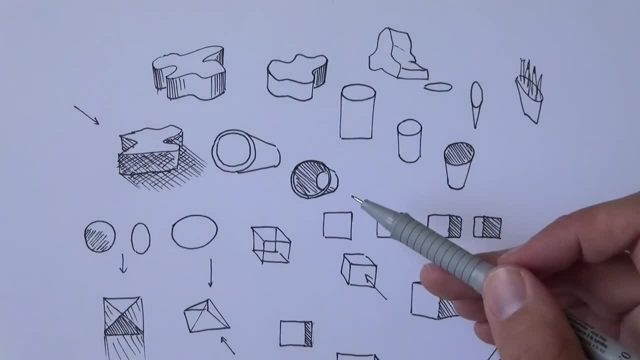 to it. This is really all just experimentation. Doing this a lot and on a regular basis will really improve your abilities to sketch and to draw what you see. Because, again, the basis for buildings is this: It's the cube. So if I see a building and I want to sort of draw it, or even 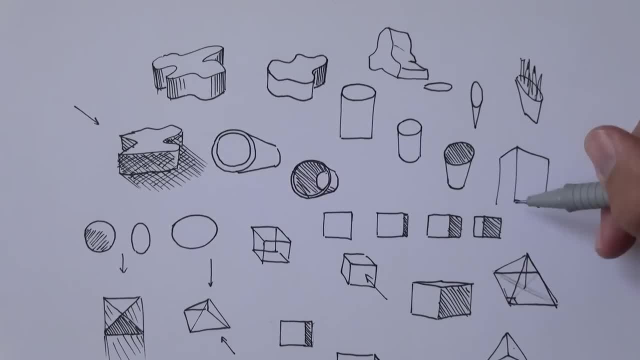 even as a preparation for a watercolor painting. that's basically sort of a cube, a cube, elongated cube, and with windows, with some more details. You can see here. maybe there's an awning here, maybe there's a restaurant at the bottom, but the concept stays the same. It's just 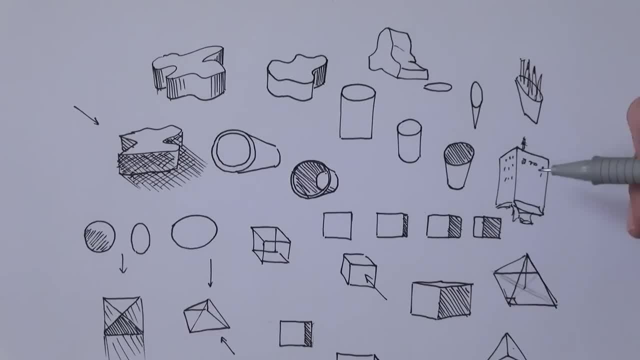 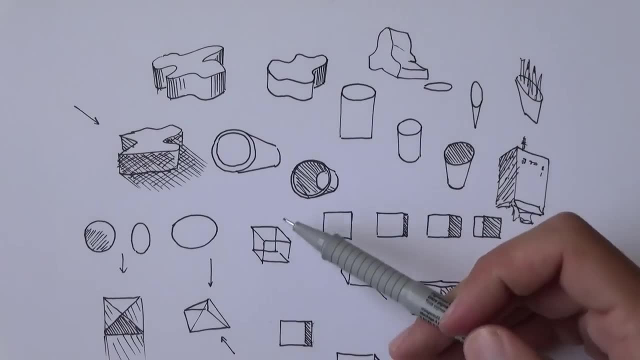 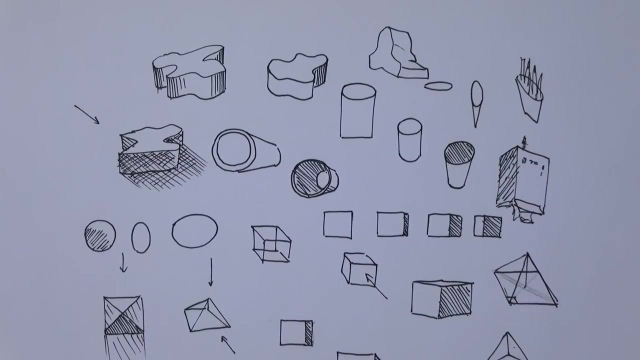 this sort of a building. there's an antenna, whatever it is, and it's just so simple once you get the sort of basic shapes to it. okay, Now, I went through a lot in this video, so what I'm curious to know is, if there's anything you want me to dive even deeper, I want you to let me know. okay, maybe you want us to sort. 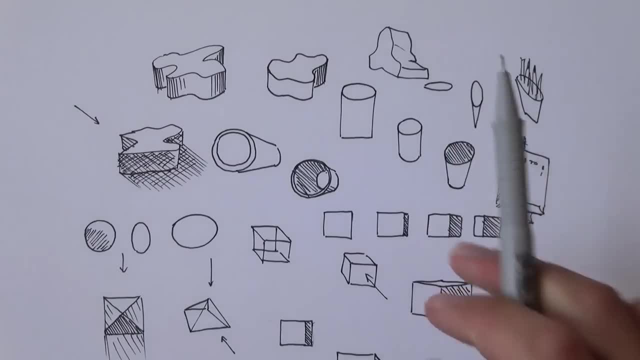 of analyze the cube on many different angles and just zoom in on that. maybe the pyramids, maybe this weird sort of exercise, maybe the shading part. Let me know in a comment below if you're you want to know more about any of these specifics. okay, I kind of dumped a lot of things at you, so you just 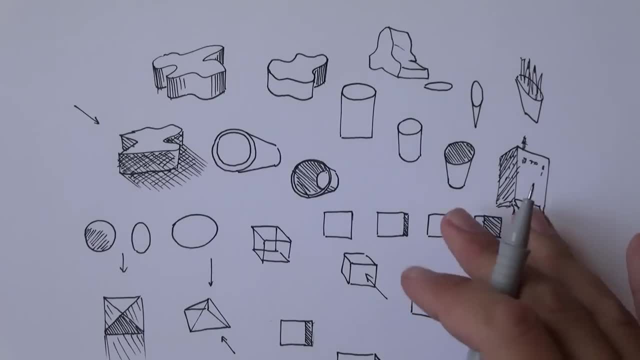 if you want something in specific or something in particular, if you want us to dive into any concept that has to do with three-dimensional shapes, let me know in a comment below. okay, I really hope you enjoyed this demo. let's change the angle and wrap up this video. okay, friends, here are all. 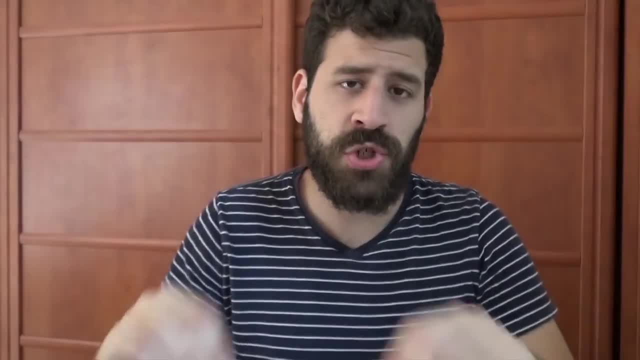 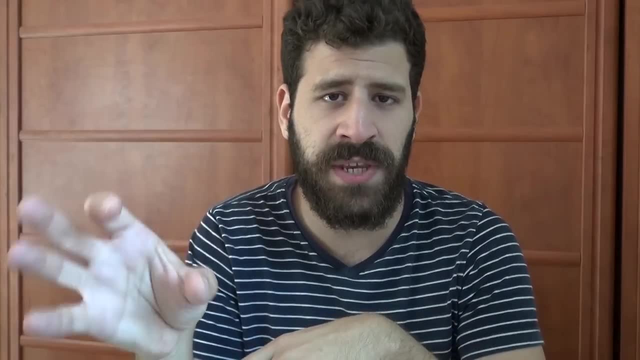 of our little doodles here. I hope you enjoyed this video. and again, as you saw, I went through a lot and little doodles here. I hope you enjoyed this video. And again, as you saw, I went through quite a bit of things here. If you want me to make a specific video on one topic, or even just, 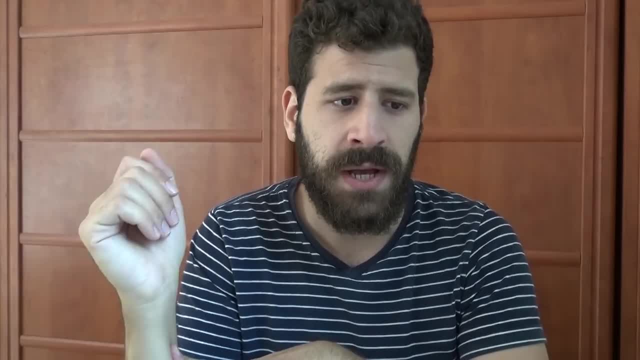 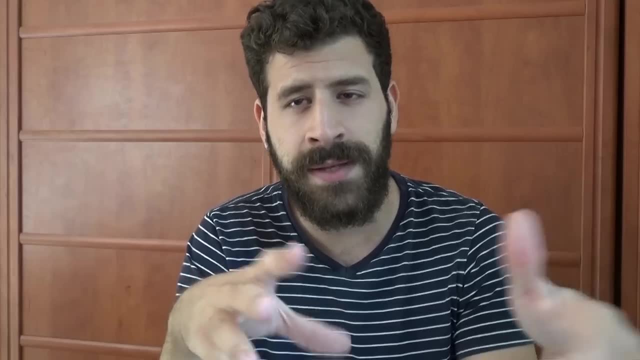 one specific shape, like the cube, or like a pyramid or maybe something that you want to bring up. I'll be happy to do so And we can sort of really analyze it more deeply and really figure out things together on how to portray it in different angles and different situations. and 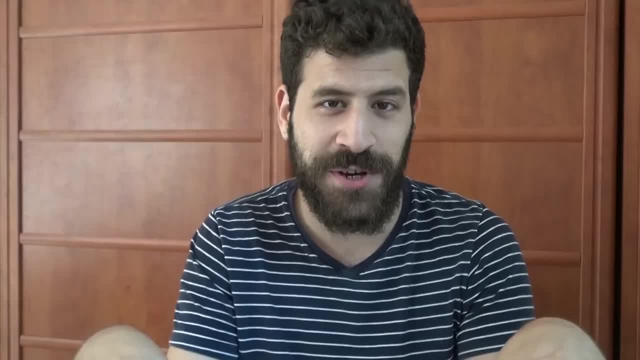 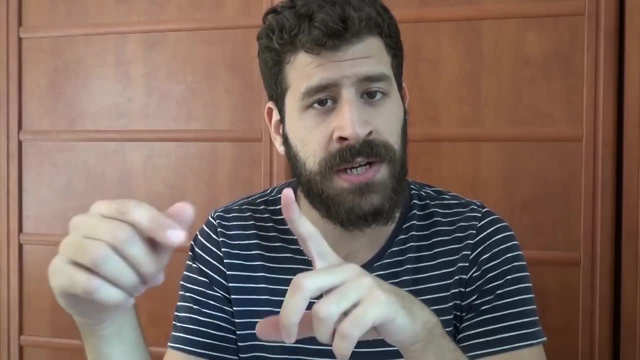 maybe even different light conditions. Okay, so I really enjoyed making this video for you. I hope you enjoyed it as well. If you enjoyed it, don't forget to subscribe here on YouTube And also follow me on Snapchat and Instagram, where I share more things on a day to day basis, especially my